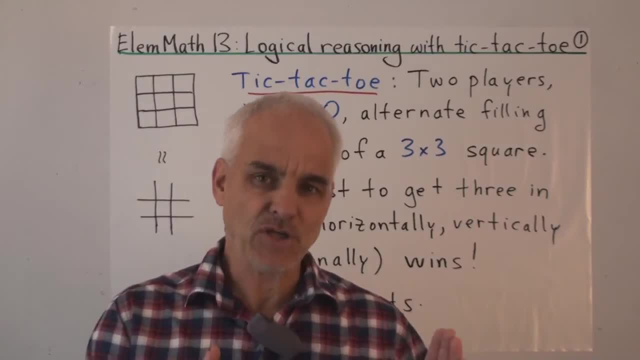 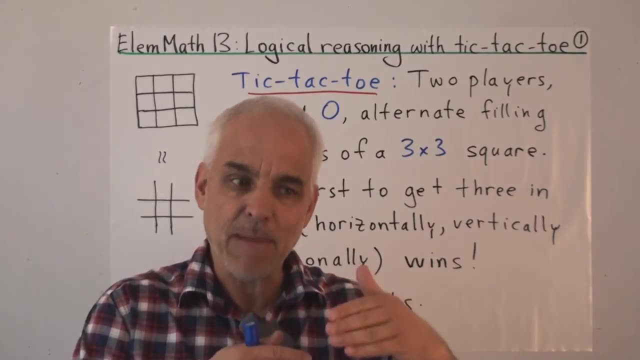 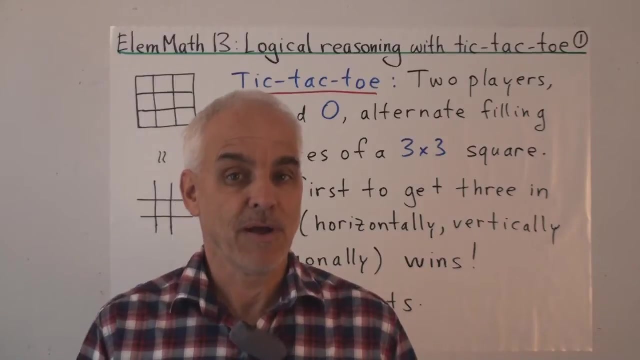 And especially, we're interested in the idea of logically analyzing it and the idea of developing a strategy which is not just short term but maybe looks ahead a few steps. So the general orientation that we're having here can be applied to a number of other things. 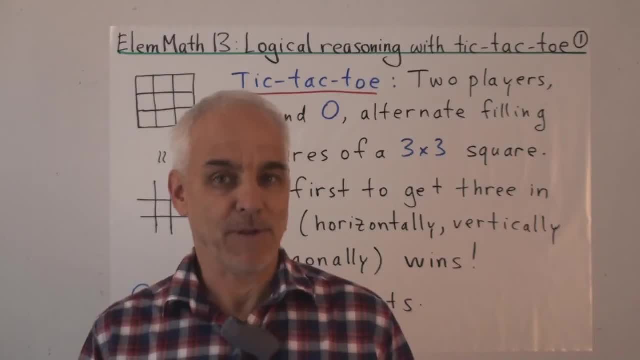 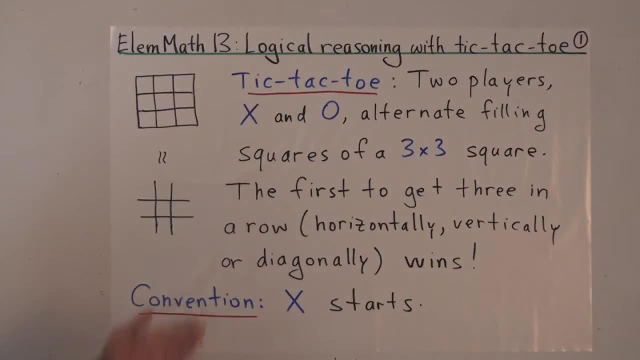 And at the end I'm going to suggest some other games that you might want to play around with. So tic-tac-toe is a game played with two players, and they're usually called X and O, And what they do is they play in a square, a 3x3 square, and they alternate, filling the squares, these little squares inside this 3x3 square, with either X's or O's. 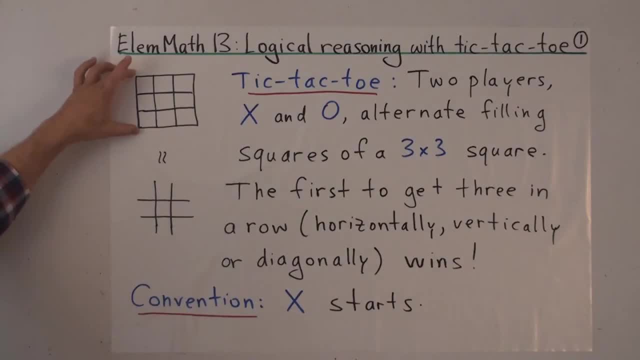 Now it's usually more common to replace this square here with a more abbreviated version like this, where we don't actually have the outside boundary, But there's still nine little squares here that have to be filled with X's and O's, And the idea is that the first person to get three in a row wins. 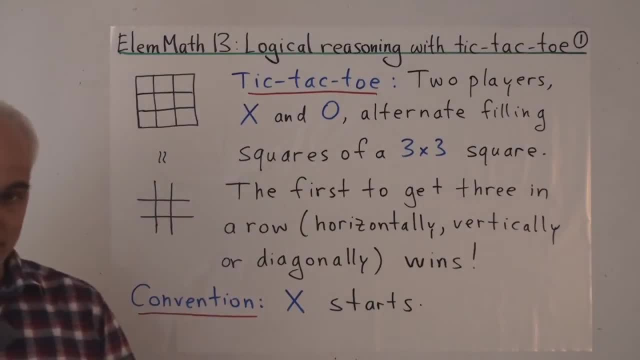 And three in a row means three either horizontally in a row or vertically in a row or diagonally, Meaning in this area This diagonal or this diagonal, And the usual convention is that X starts. So let's play a game. 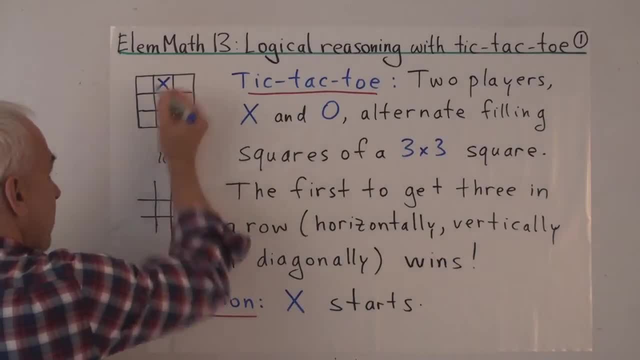 Let's play up here first X starts. so let's say X randomly plays there And then O, not having played this game before, randomly plays there, Maybe X plays here And maybe O plays here. Now X can see that O is trying to get three in a row. 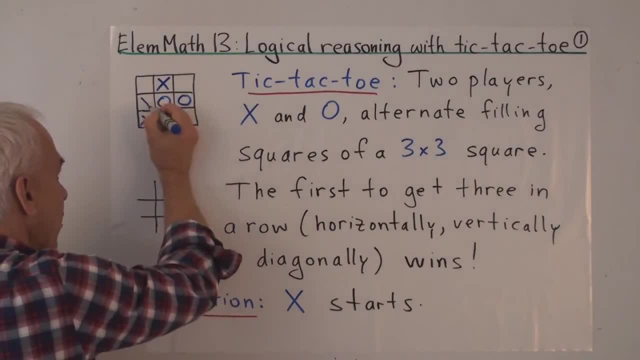 So X wants to prevent that. So X goes there And now O is thinking, well, what should I do? And then he realizes: wait a minute, I better watch out because X is about to make three in a row vertically. 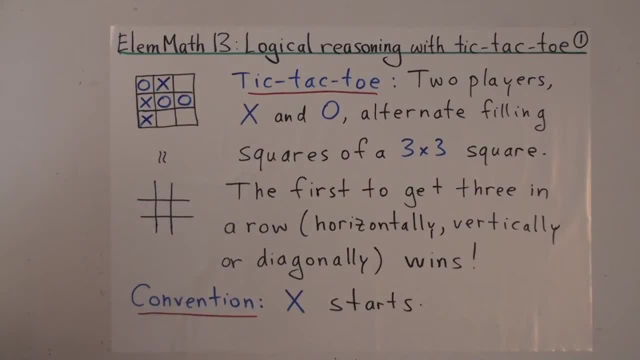 And so he goes there. And then X thinks, well, maybe I'll try to make three in a row in this direction. And then O plays here and realizes that he has just won Because these three O's along the diagonal form a three. 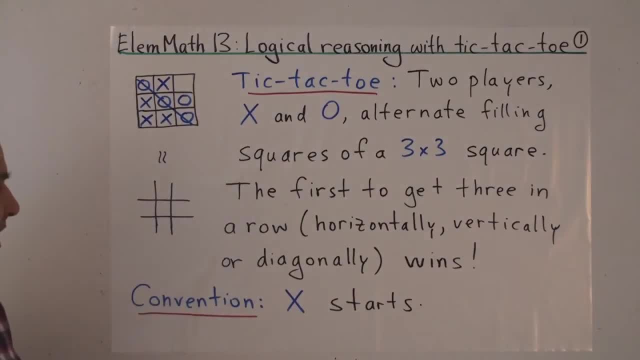 So O has made the three. He's got three in a row down the diagonal, So O wins. Let's play another game. So this time X plays here. still, This time O will play here. Maybe X plays here. Maybe O plays here. 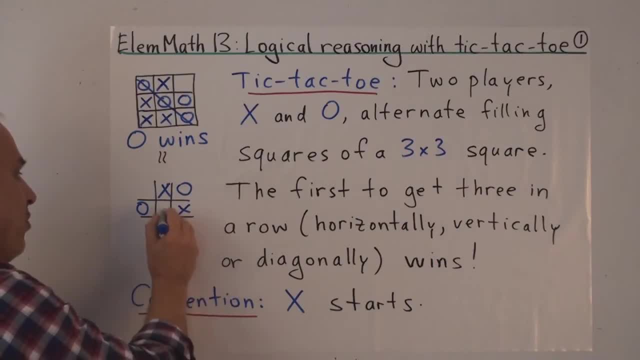 Maybe X plays here, O plays here, X here, O here, X here. Well, in this case, the game has finished. There's no more room to play. Neither player has gotten three in a row, So this is a draw. 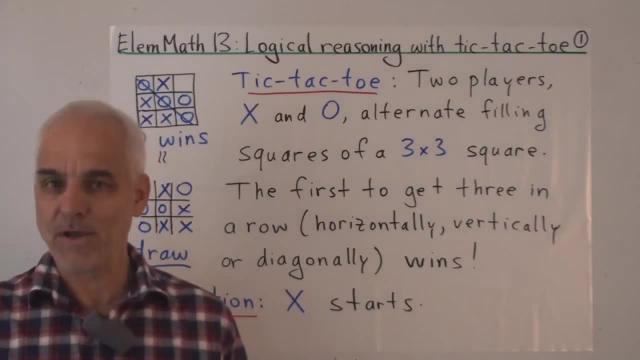 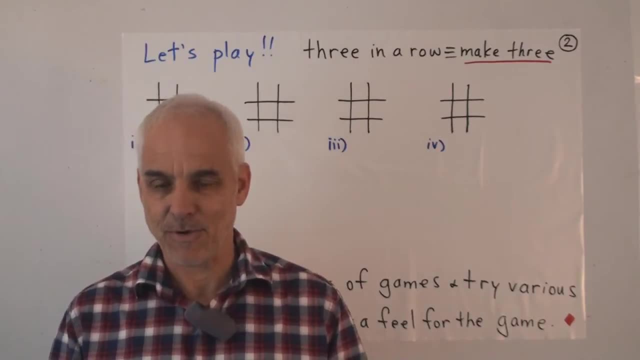 So the game can end either in X winning or O winning or a draw. I am confident that most of you have played this game before And you probably have a reasonably good idea how it works, But let's anyway just develop some intuition by playing some more games. 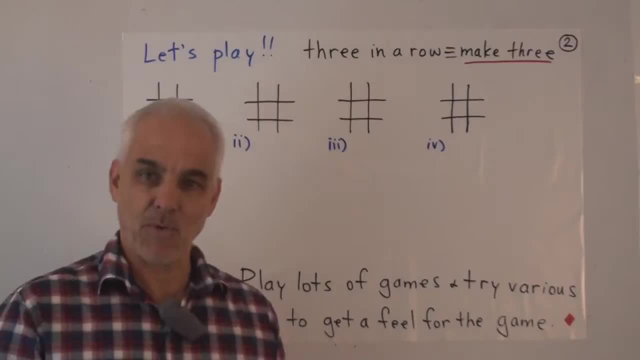 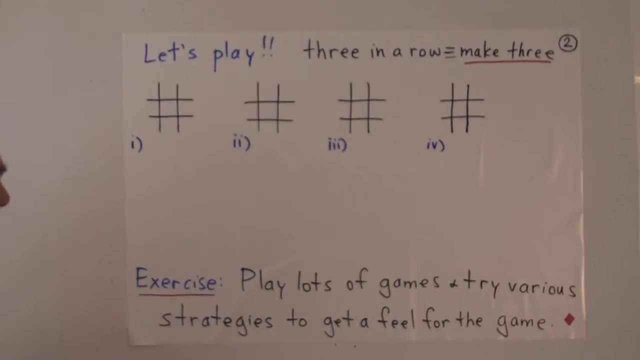 It's a good way to become familiar with a mathematical or logical situation. It's to explore it a little bit. So let's play a couple of games. Game number one: This time X is going to think: well, maybe the center square is the most important. 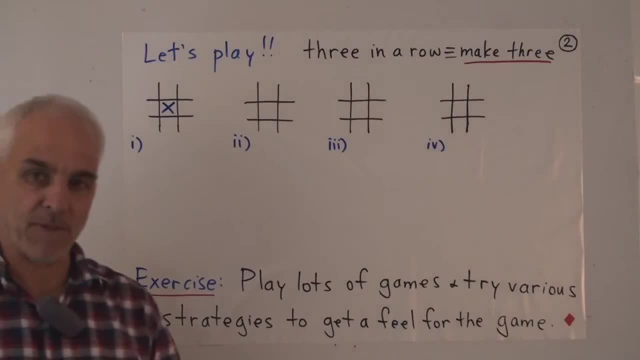 Because there's more ways, it seems, of making three in a row with the center than with the other ones. And then O will play, perhaps with the corner, And then X is going to play here And O plays here, And he doesn't realize that X is about to make three. 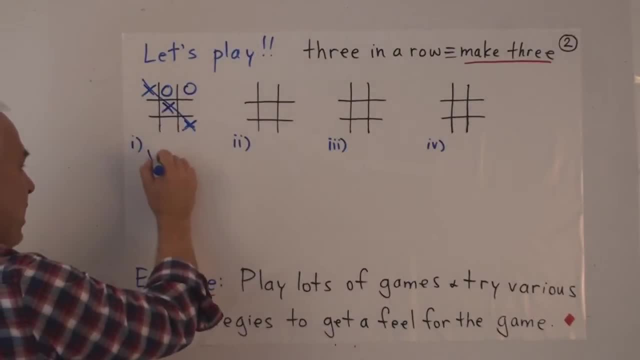 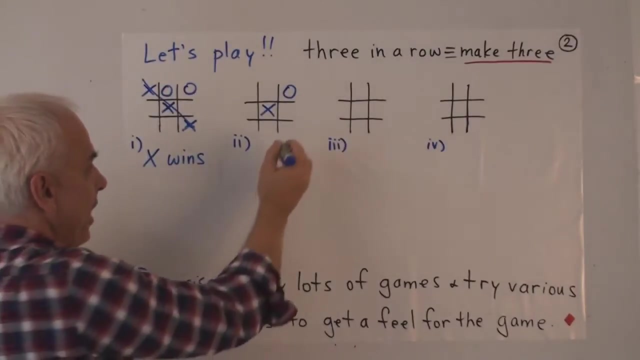 And so X makes three along that diagonal And X wins. That was not such good play on O's part. They play again. So this time X still plays in the middle And O plays outside here, And he's going to play a little bit differently. 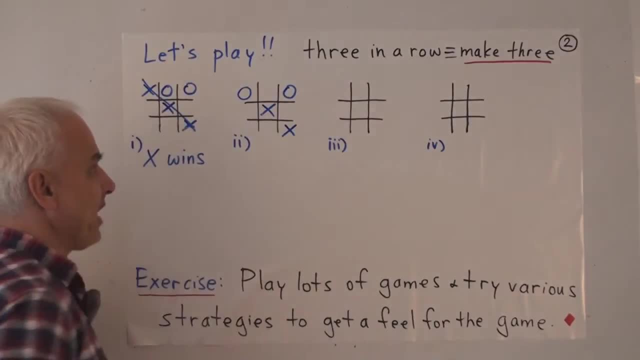 Now he realizes that he better answer these two X's, because X is making a threat here. He's threatening to make three in a row. And now X decides: ah, this is a clever play, because now I can make three in a row either this way or this way. 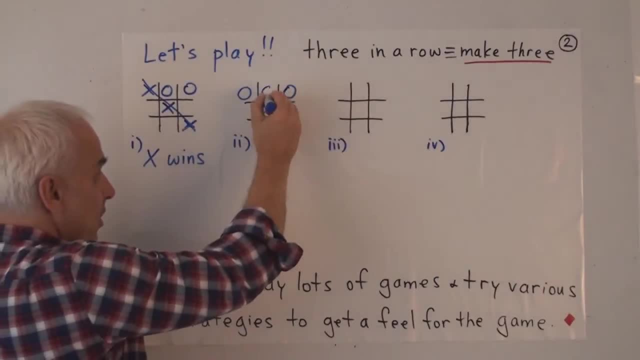 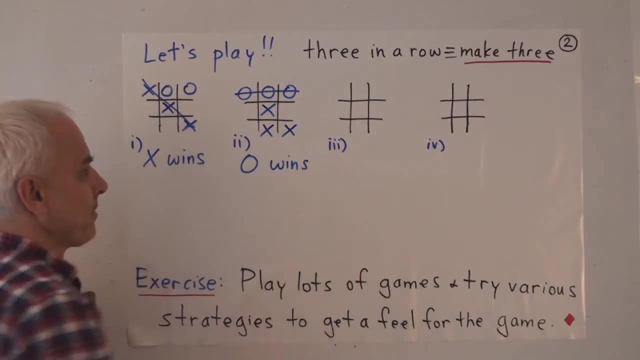 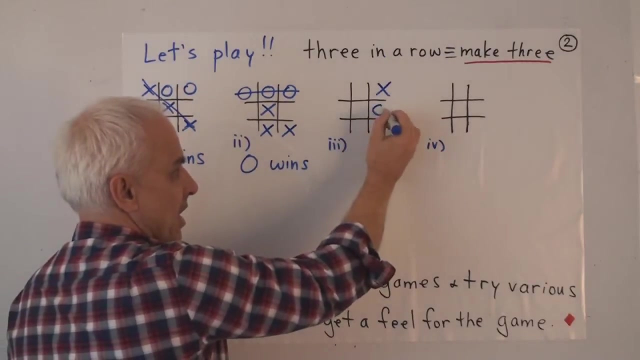 That seems like a good idea, Except that he forgot that O could actually finish by making those three in a row there. So here O wins. X is going to try something different this time. Maybe play in the corner And O will play along the side. 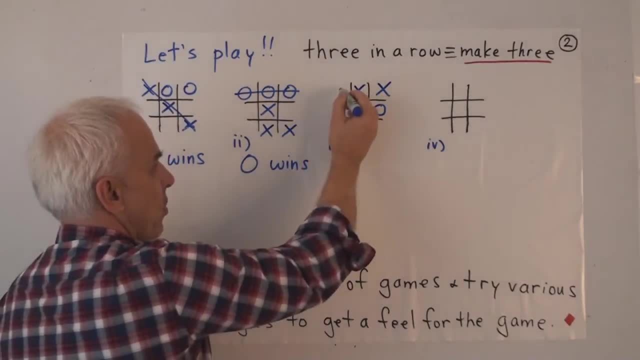 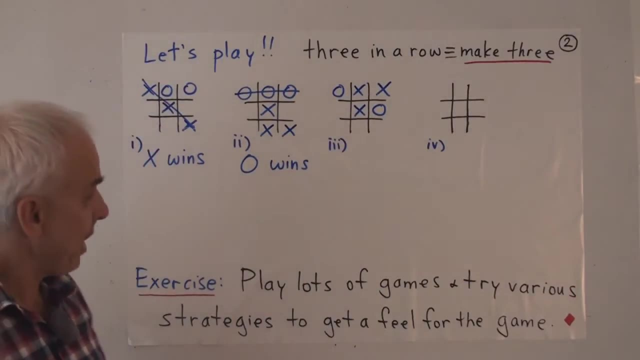 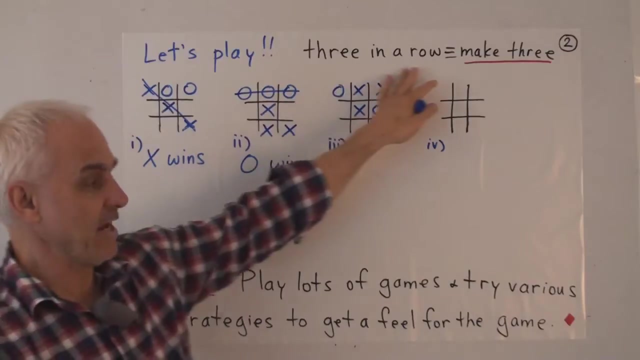 And perhaps X will play here And O will play here, And now X plays here, And now X sees that he's in a happy situation because he's threatening to make three along that vertical row. When I say make three, it's just a short form for saying 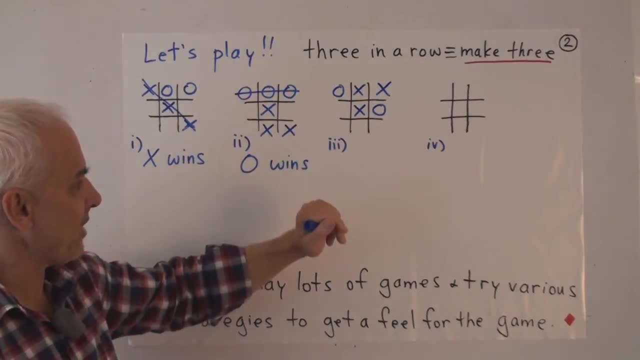 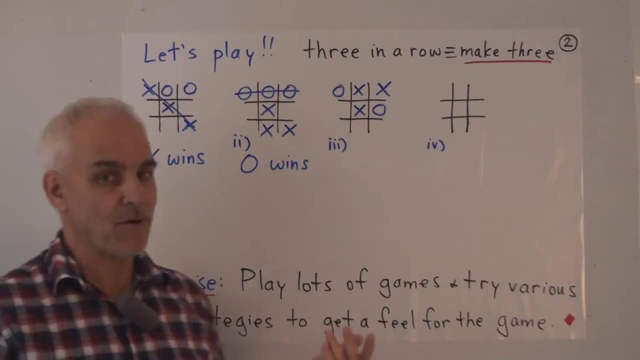 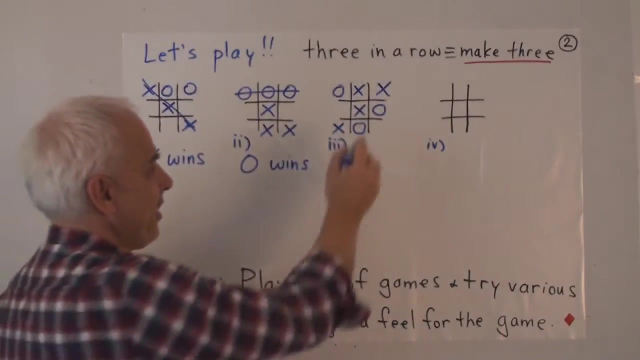 make three in a row. So X is threatening to make three along that vertical row and also along that diagonal. So O cannot play in those both places at once. He can only play in one of the places, in which case X can play in the other. 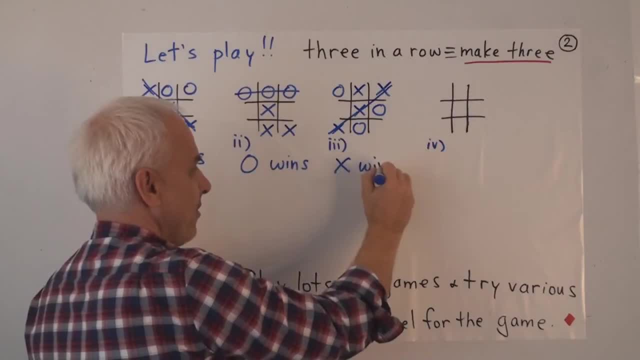 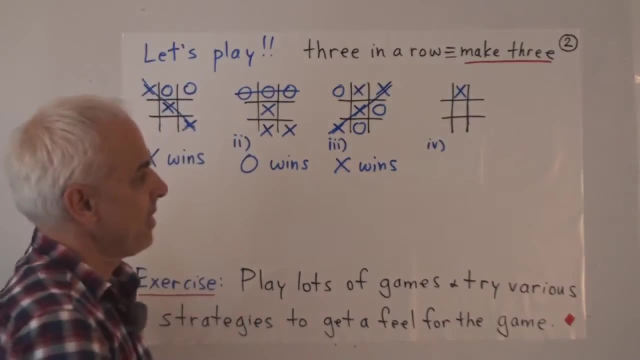 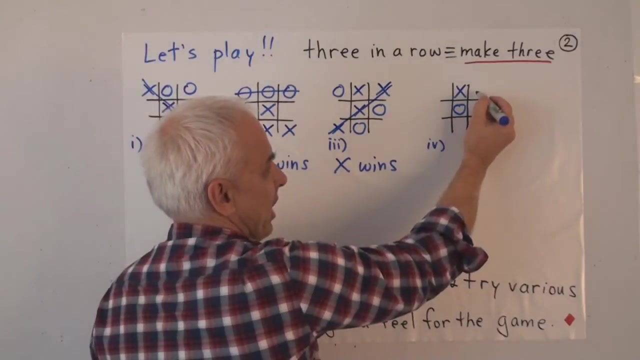 and make three in a row. So X wins. And one more try. Let's have X starting on the side this time. Maybe O will take the center square And maybe X will play here. let's say O will play here. 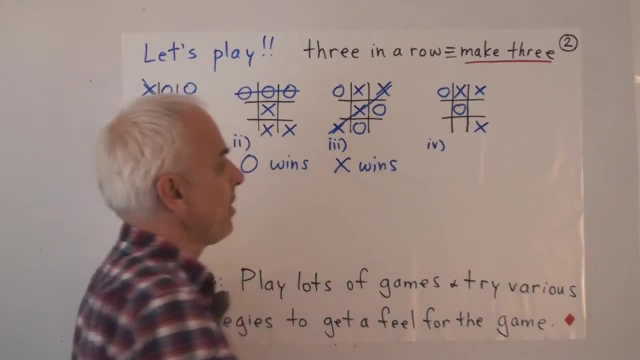 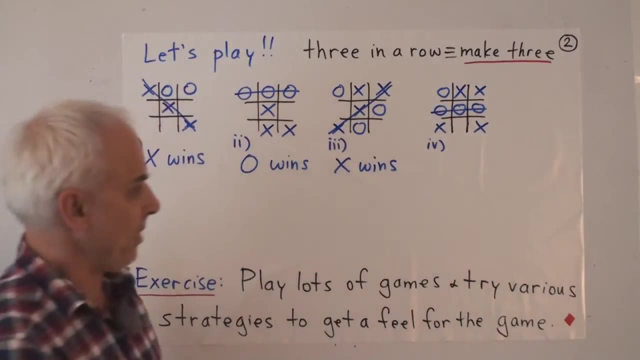 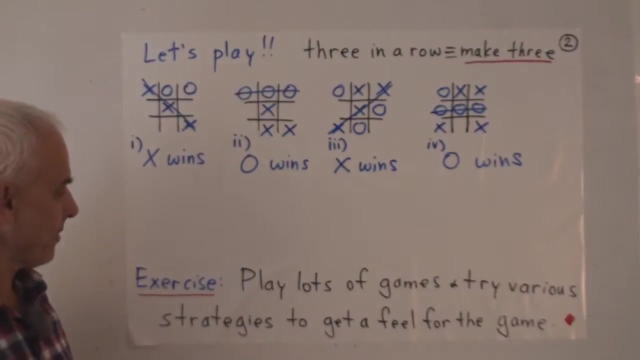 And X will play here. O will play here. X plays here. Whoops, He didn't see that O was about to make three in a row, So O wins this time. Alright, so your first exercise is just to play some games. 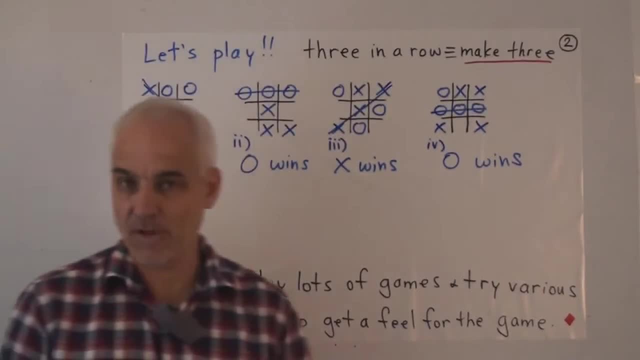 or play lots of games and try various strategies to get a feel for the game. How should one play X's and O's? What's a good strategy? Does the first player always win? How should both players play? It seems as if there's something asymmetrical. 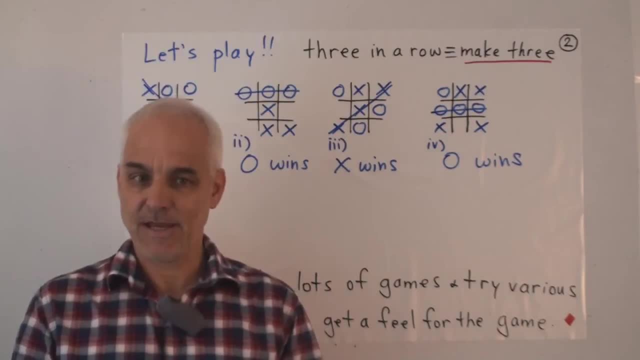 because the first player sort of has an advantage: He gets to place his X before the other one Gets his O. So there's more X's out there on the board to make three in a row with. And that's true. The first player does have a significant advantage in this game. 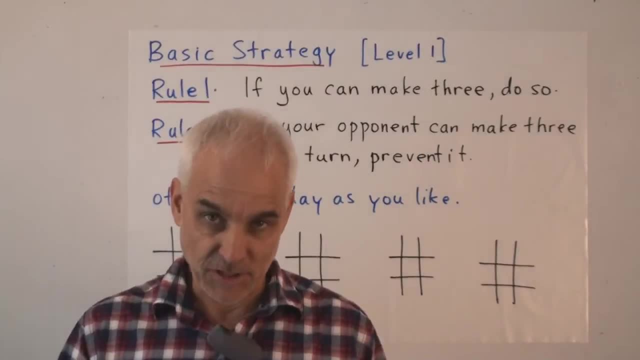 It's not a fair game. Of course, one strategy for playing this game is simply to play randomly, To play wherever you feel like playing. That's obviously not such a good idea. After you play a little while, you realize what the basic strategy is. 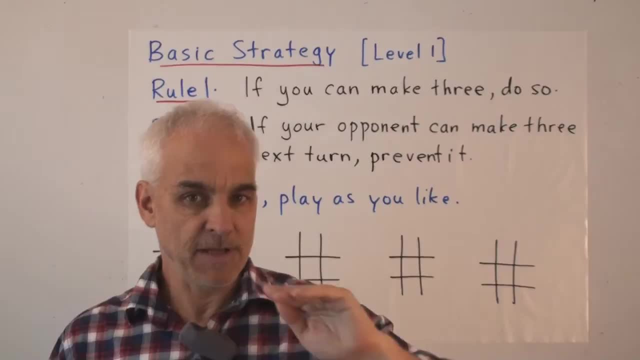 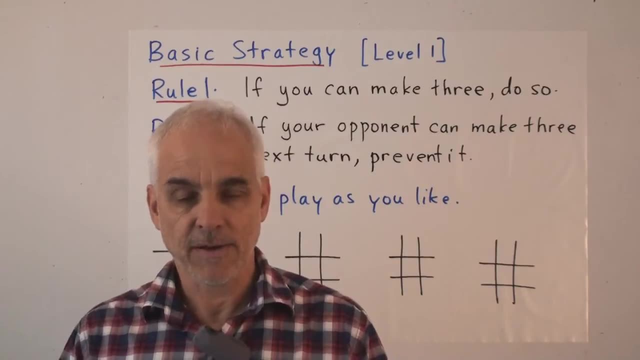 This is sort of level one strategy. We're going to see that there are a number of different levels of playing or different levels of understanding this game. The level one strategy is what I think any kindergarten or year one student is going to discover after they play this game a few times. 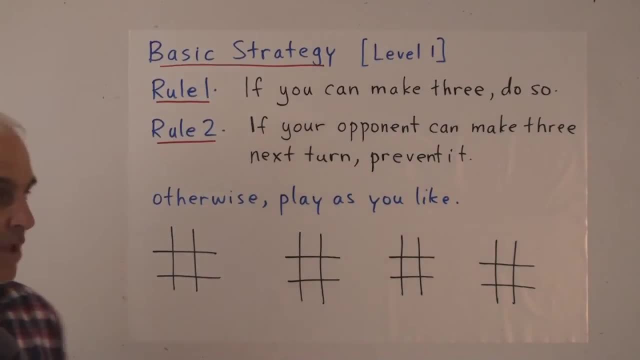 The strategy has two rules. The first rule is that if you can make three, do so. If it's your turn and you're looking at the board and there's a possibility for making three in a row, do it, Because that will finish the game right then and there. 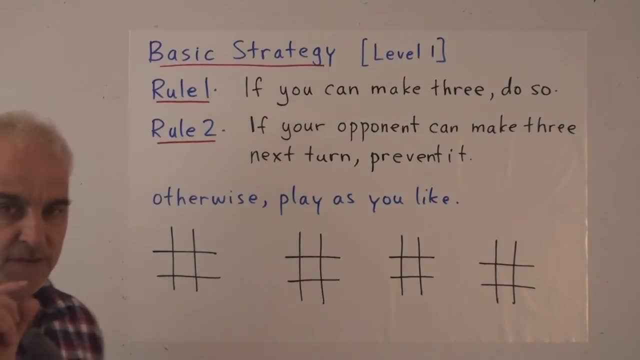 the game will be over and you will have won. So this is the first thing that one does at each turn is to look at the board and see if there's a place where you can make three. Rule number two is only to be used if rule number one doesn't apply. 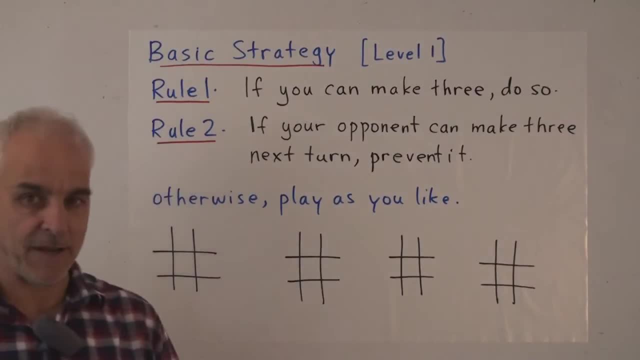 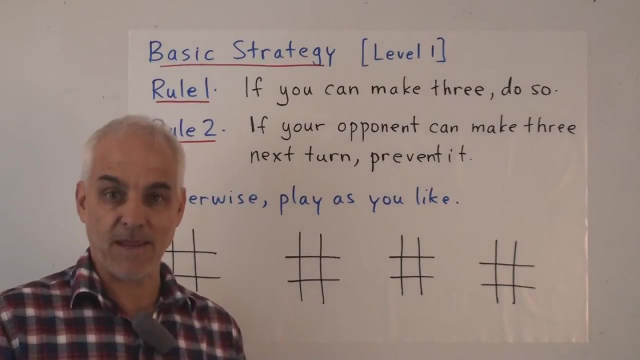 So if rule number one doesn't apply, then rule number two kicks in, And rule number two says that if your opponent can make three, next turn prevent it. In other words, it's your turn. You just looked at the board. You've just seen whether there's a way of making three or not. 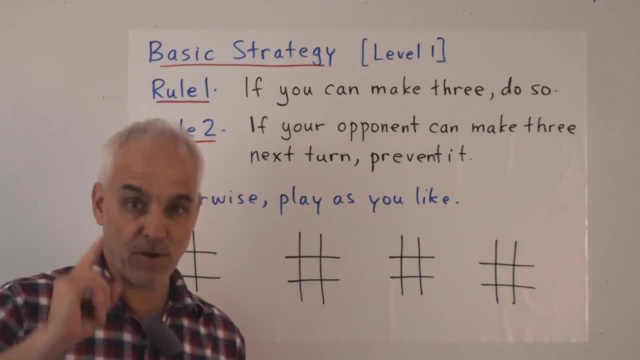 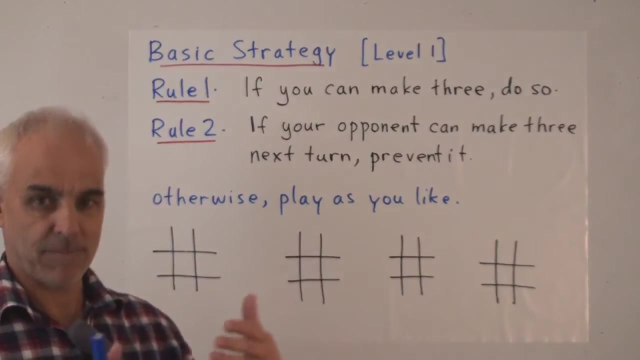 You've decided. unfortunately, there's no way of making three. So the next thing you better look at is: can the opponent make three next turn? If they can, then you must prevent it. So having these two rules in mind is already a start to having a good strategy. 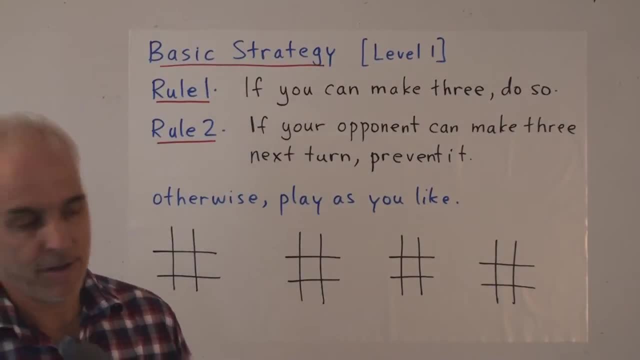 We call this the basic strategy for tic-tac-toe, So let's illustrate it in some examples. So suppose that we have a situation where we already have this board position And it's X's turn. So X will look at this board and say: 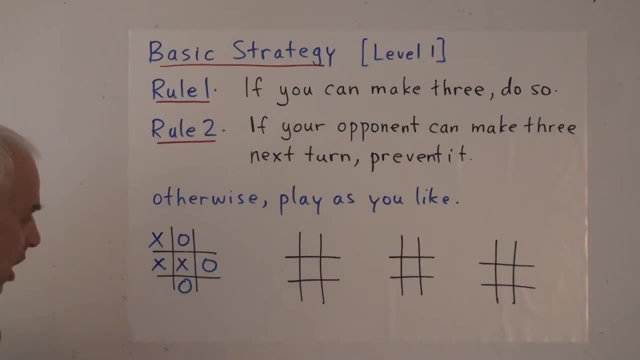 OK, there's three places I can go. Are any of those places going to make three for me? Well, this place makes three. In fact, this place also makes three, So both of these two places will be a win for X. 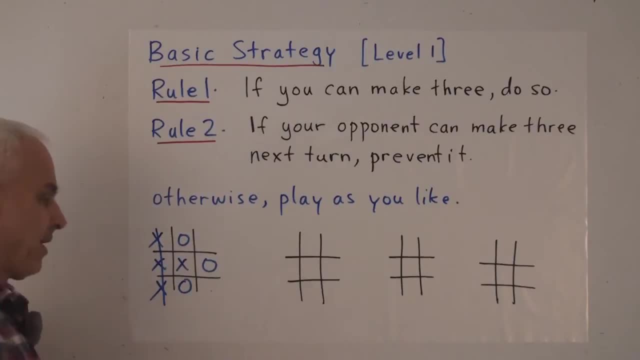 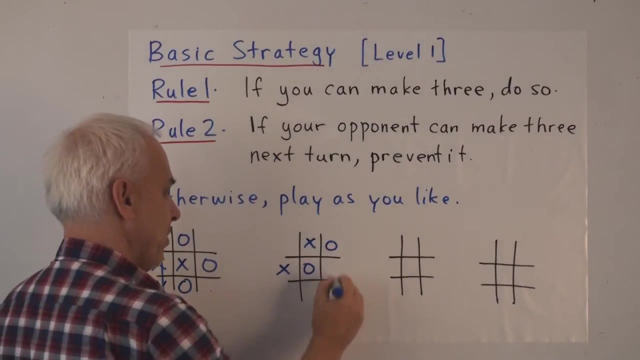 So choose one of them, make three X wins. OK, here's another situation: X zero, X zero, Just like that. let's say It's X's turn. The first thing X does is he looks. can I make three? 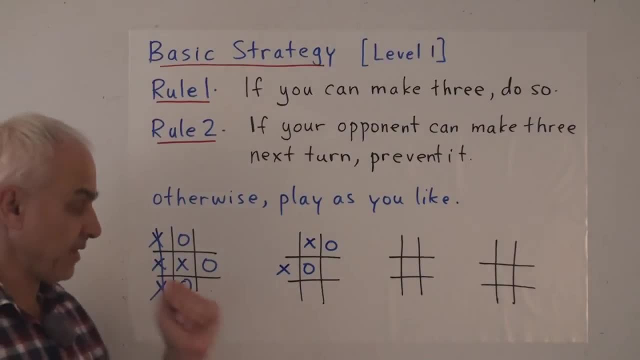 No, X cannot make three. So the second thing that X must do is look to see: can O make three? next turn? Well, yes, he can. He can play here in this corner to make three along that diagonal. So X had better play there to prevent O from playing there. 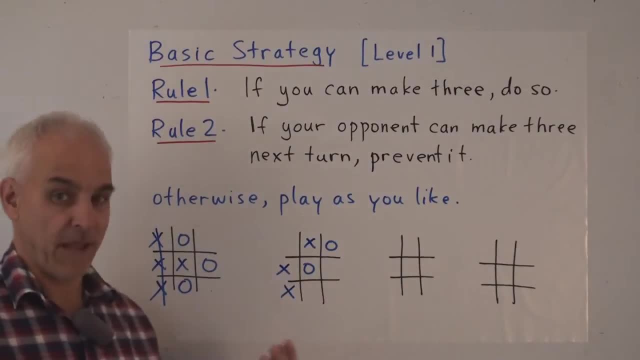 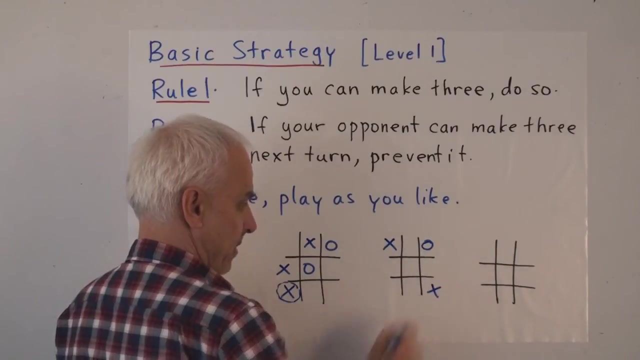 Because if he doesn't, then O is going to play there and the game will be over and X will have lost. So that's the move that X must make. How about for O? Suppose we have this situation. In this situation, it's O's turn. 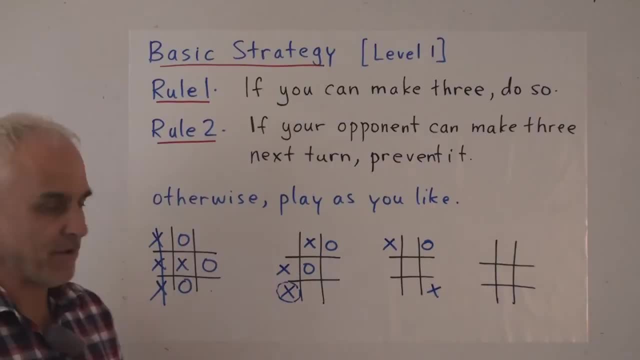 O looks around, can he make three? Well, he can't. he's only played one so far, But he can prevent X from making three, and so he does so. So he's pretty well forced to play there. And now X looks and says: well, what can I do? 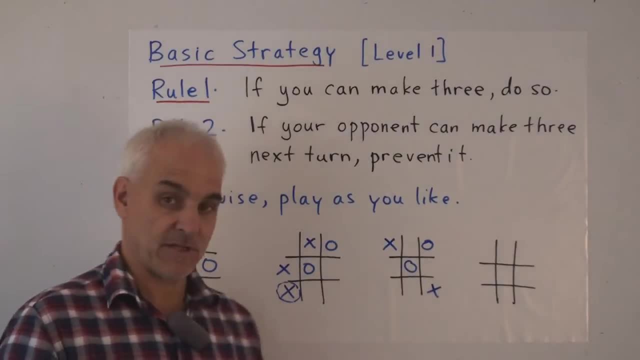 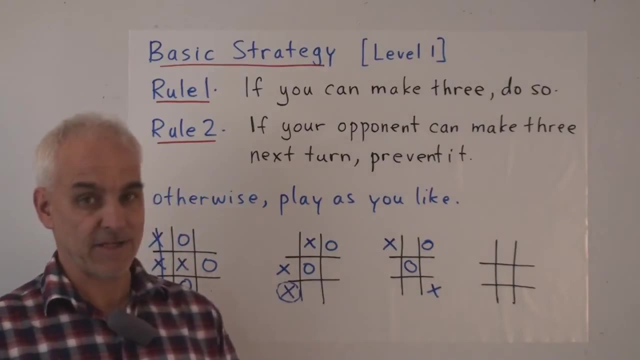 Can I make three? Well, he can't make three because O has just gone in the only place where he could have made three. And so he asks: well, if I can't make three, can O make three next time? Yes, O can make three next time. 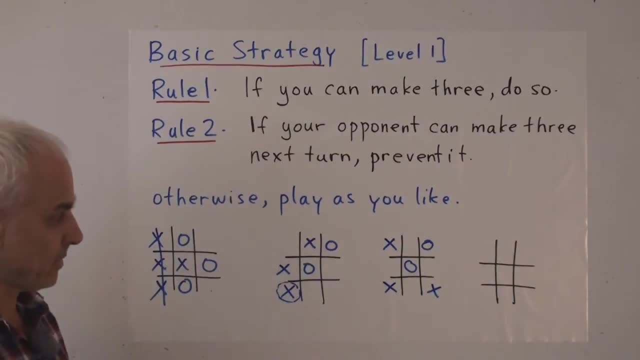 Right there. so X has better go there and prevent him. And now it's O's turn. O looks, says: well, can I make three? No, he can't. Alright, can your opponent make three? Yes, your opponent can make three here. 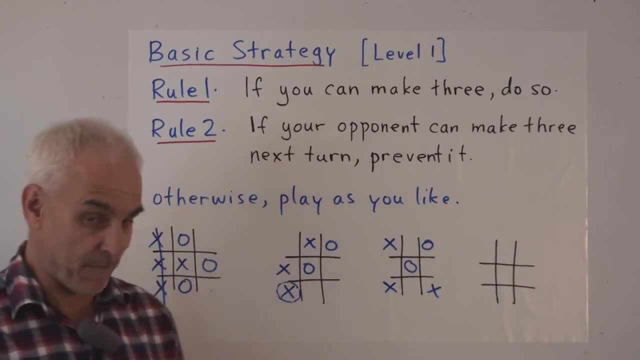 And you can see that there's a row waiting to be made here by X. So O's going to prevent it. Now it's X's turn. First thing that X does is he should not look at these two O's. Okay, here are the two O's. 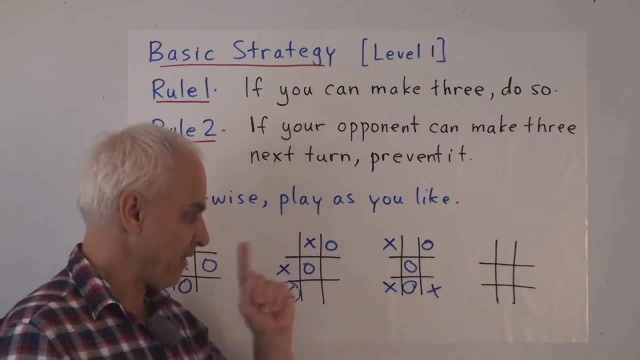 The O is about to make another third O there, But the first thing that X should do is look and say: can I make three? And X can make three, so he will play there and he will win. Let's play a more full game. 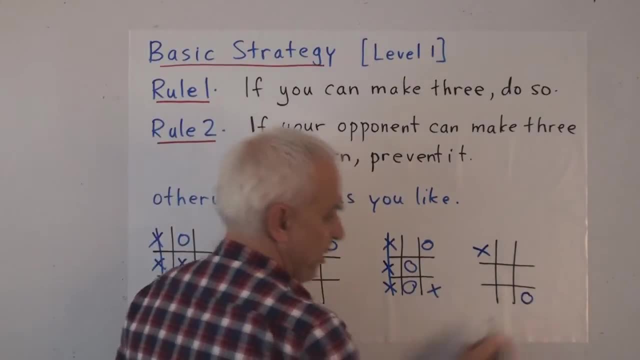 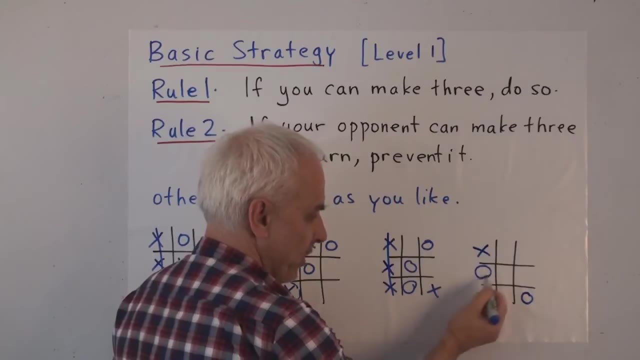 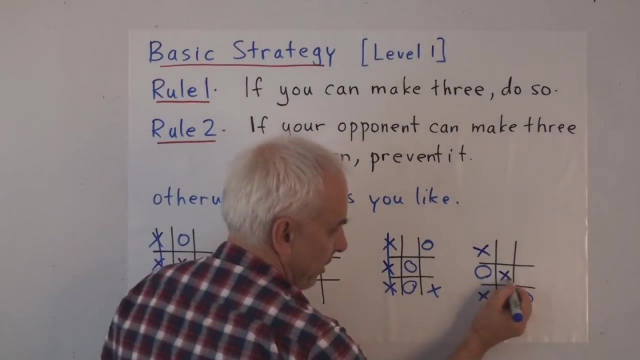 So X plays here. Let's say O plays here, X plays here, O must play here. No choice. That's rule number two. Now X has some choice. Okay, maybe he'll play here. That's not, in fact, the best move, is it? 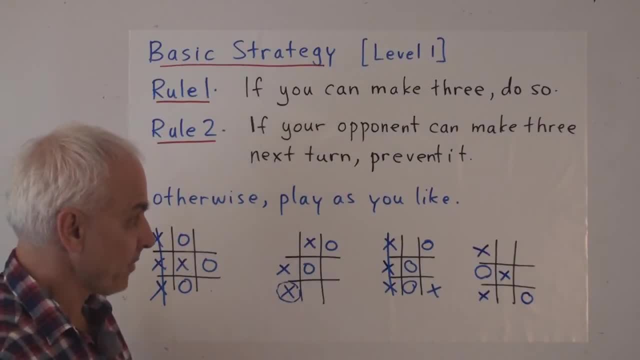 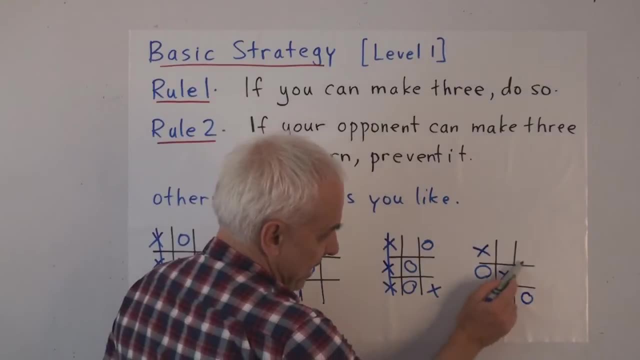 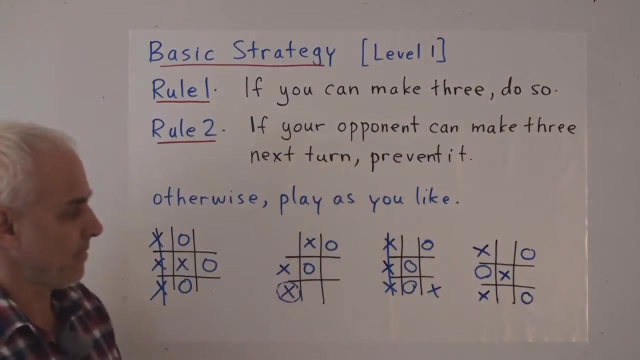 But suppose that he does, Then it's O's turn. Can O make three? No, Can O prevent his opponent from making three? Yes, he can, because X has a diagonal three coming up there. O had better prevent it. Now it's X's turn. 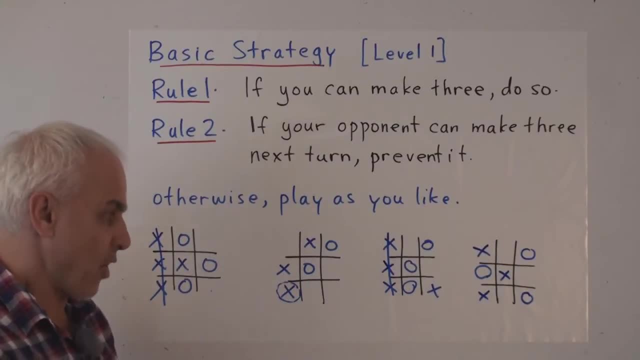 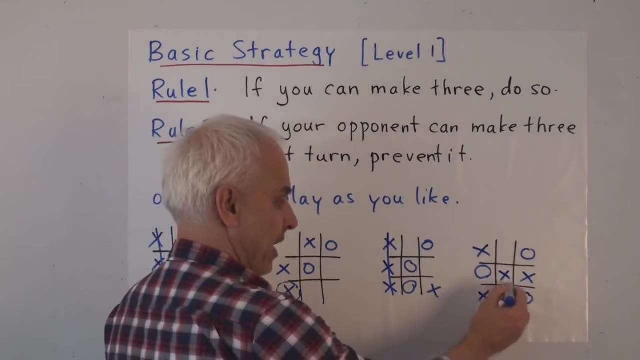 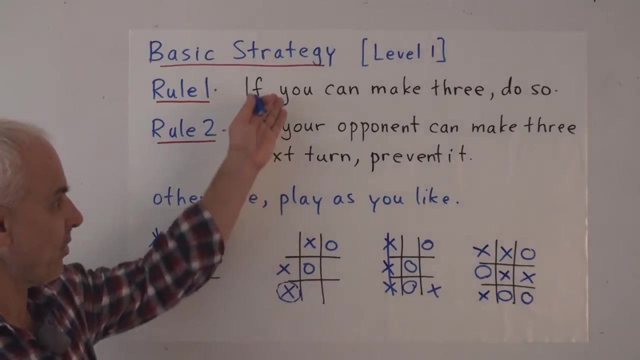 Can X make three? No. Can he prevent O from making three? Yes, so X has to play here, And then it doesn't matter what O plays next, And what X plays next is going to be a draw. So that's the kind of strategy that we can get at with this basic strategy. 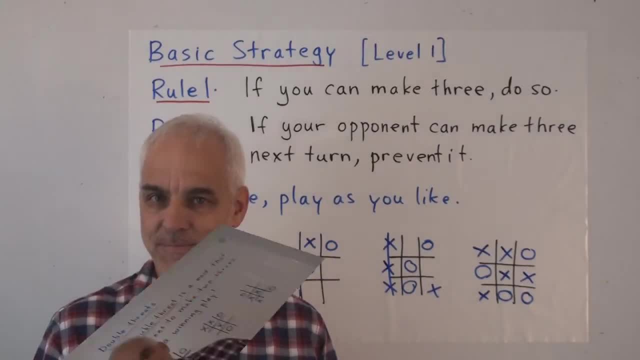 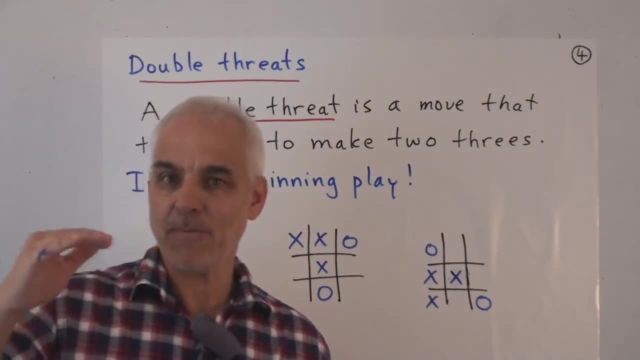 This is level one: understanding of what goes on. So once the young person has understood how to play the basic strategy for tic-tac-toe, then it's time eventually to move up to the next level, which is understanding the idea of a double threat. 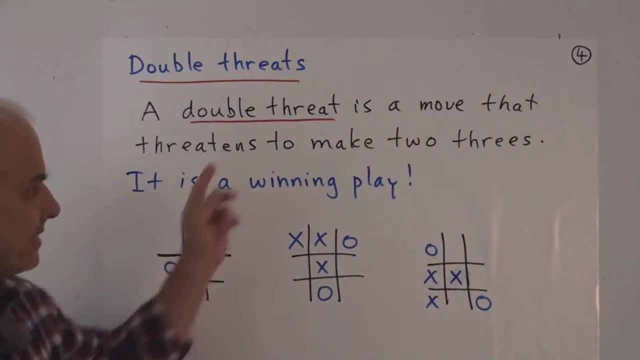 So what is a double threat? It's a move that threatens to make two threes. It doesn't actually make a three, but it threatens to make not one but two different threes. So, for example, in this situation, it's X's turn to play. 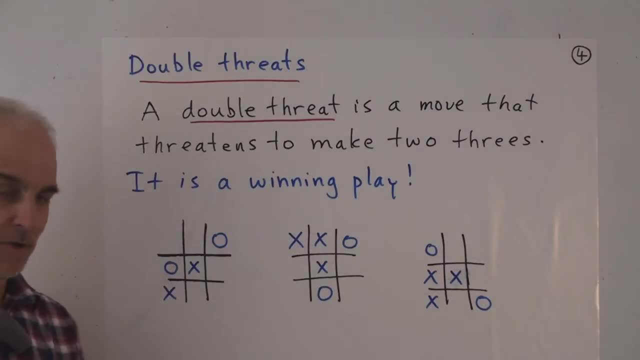 By the way, we can tell that because X always plays first and there are two X's that have been played and two O's that have been played, So it must be X's turn to play. So where can X play? Well, of course, he cannot make a three in a row directly. 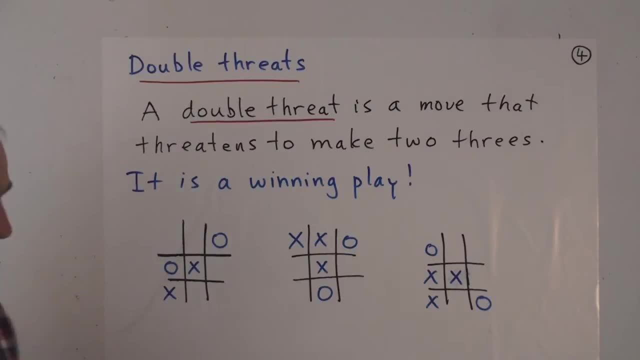 and he doesn't have to worry about O making a three next turn. so he kind of has a free move to do whatever he wants to, And he has a number of good possibilities. Here is one of them. Have a look at this move. 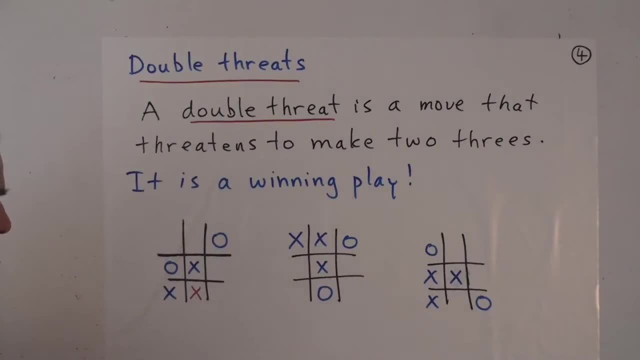 That's a double threat by X, because it threatens a three in this direction and it also threatens a three in this direction. O is going to be able to prevent one of those threes, but not both of them, So O plays here. 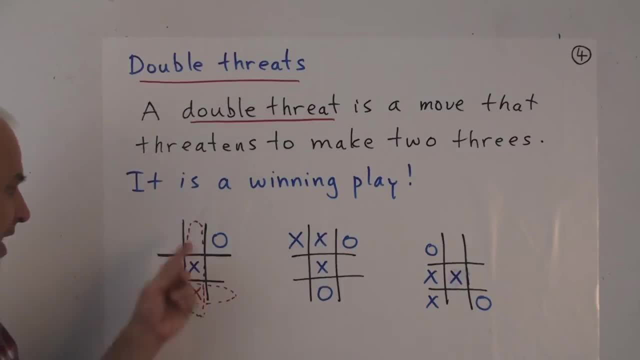 In that case X plays there and wins. On the other hand, if O plays there, then X plays here and wins. So this is a double threat move and it's a winning play. There's another double threat play in this situation. 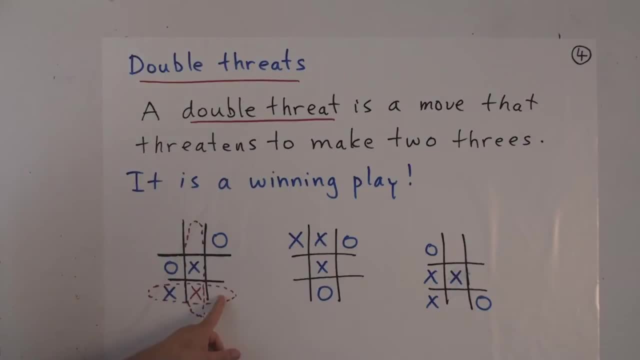 If X plays, not here, rather, but in this corner, then you can see- I hope- that that's also a double threat, because it still threatens a three in this direction and it also threatens three along that diagonal. So X was in a happy position of having two double threats. 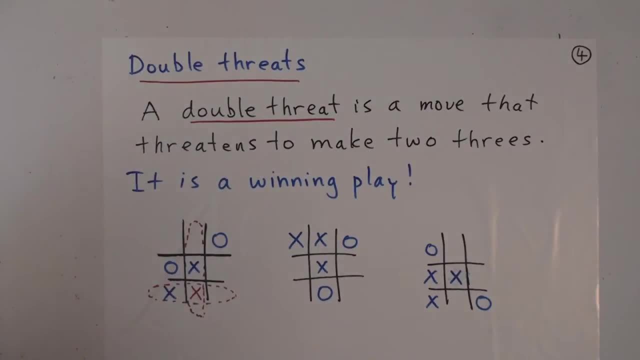 that he could find in that position Here. in this situation, X has played three times and O has played twice, so it's O's turn. Alright, what should O do? So, according to rule one, first O looks to see if he can make three. 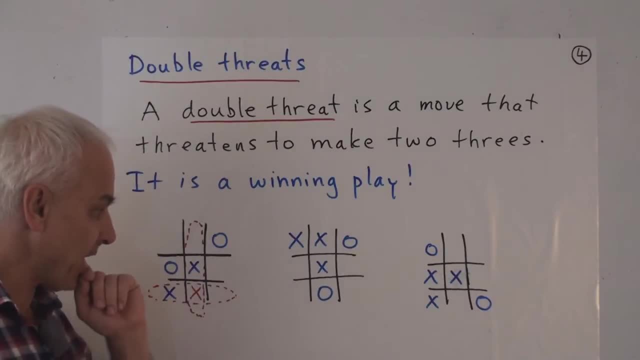 He can't. Then he looks to see: well, can X make three? Yes, actually X can make three right along there. So in fact O has no choice, He has to play here. But after he's done so, he realizes. 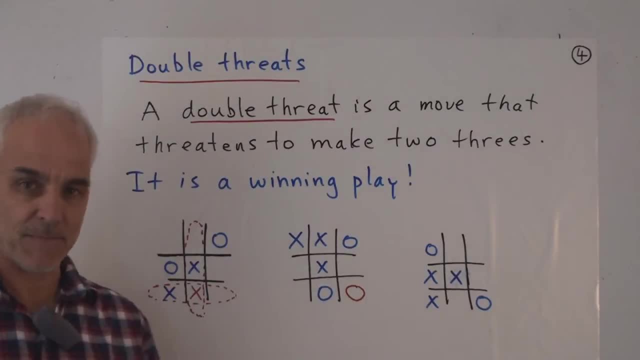 that was actually pretty fortunate, because that's actually now a double threat. It's threatening to make a three in this direction, and it's also making a threat to make a three in this direction, And so O is going to win. It doesn't matter what X plays. 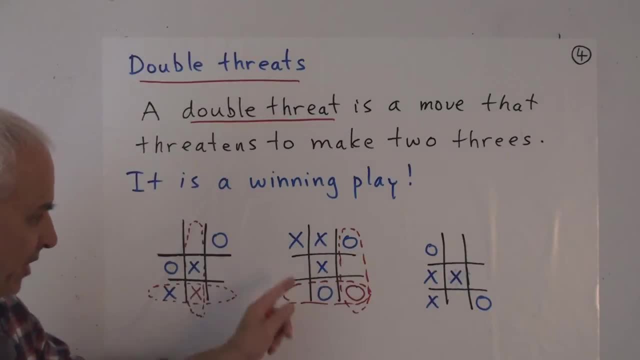 If X plays here, O will win there. If X plays here, then O will win there. So here we have X winning and here we have O winning. How about in this situation? X has played three times, O has played twice, so it's O's move again. 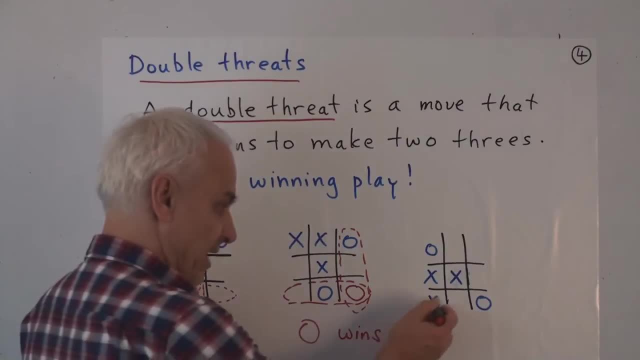 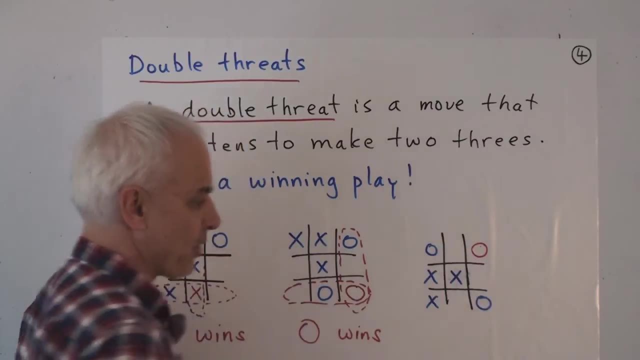 And again O only has one choice, because he has to prevent this three diagonal of X along here, and so he has to play in that corner. And it's the same kind of thing, but it's a little bit different configuration. Now he sees that he's making a double threat along this row. 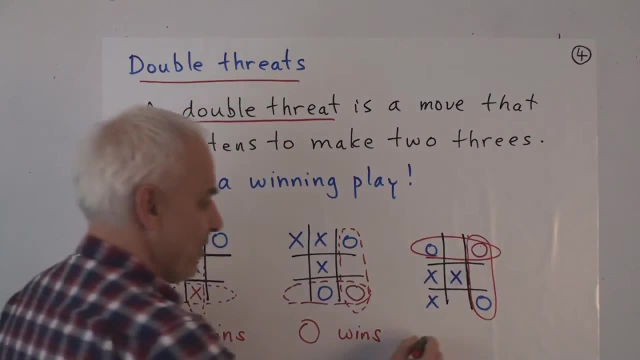 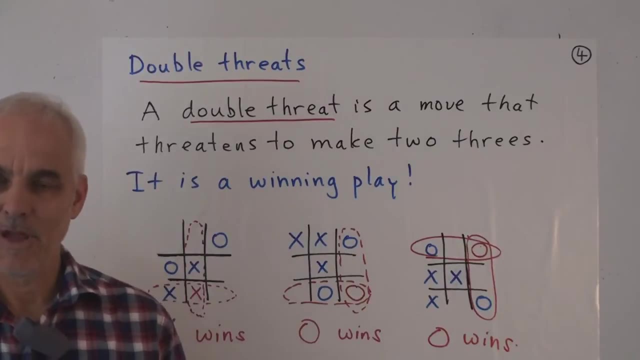 and this column. so again, O wins. So this is the next level of play is to recognize that, after you've got the basic strategy down, you want to look for double threats. Alright. so now let's introduce the next level of strategy. 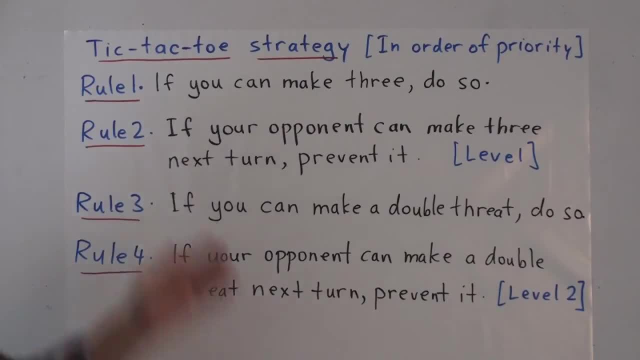 So now we have four rules. We have the two rules that we started with, and now the third rule is that if you can make a double threat, do so. And the fourth rule is that if you can't make a double threat, look to see if your opponent can. 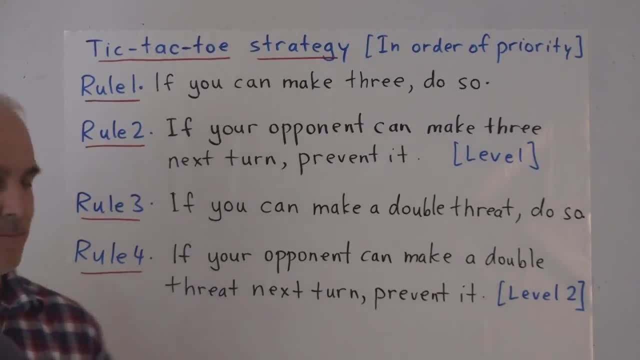 And if he can prevent it. So now we have four rules for tic-tac-toe strategy. This is now level two kind of understanding. First rule: if you can make three, do so. Rule two: if your opponent can make three, next turn, prevent it. 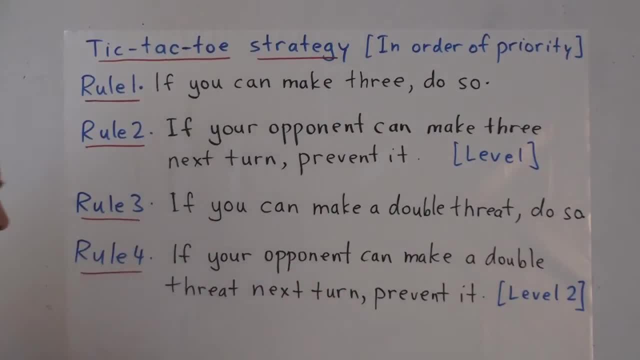 Third rule: if you can make a double threat, do so. Fourth rule: if your opponent can make a double threat, next turn, prevent it. And we check these things sort of one at a time. First we check whether we can make three. 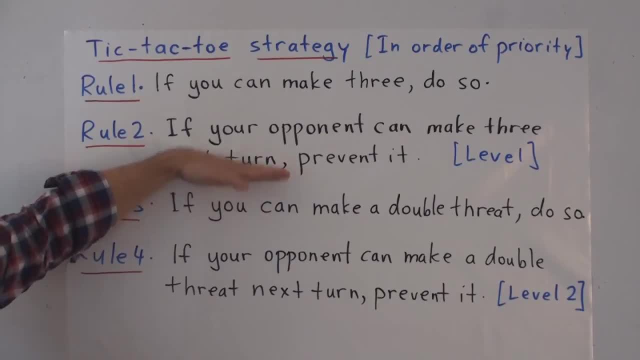 Then we check whether the opponent can make three- These are direct making of three- Then we check whether we can have a double threat which ensures that we'll be able to make a three next time, And then we check whether the opponent has an opportunity. 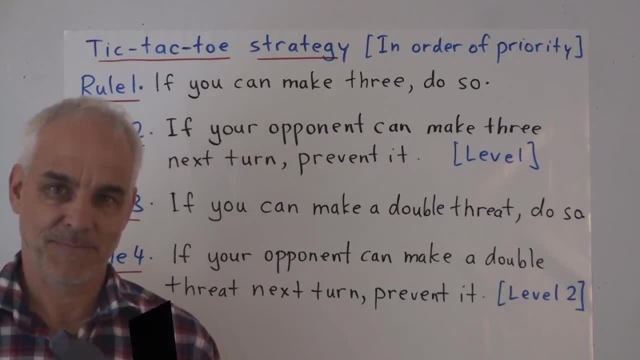 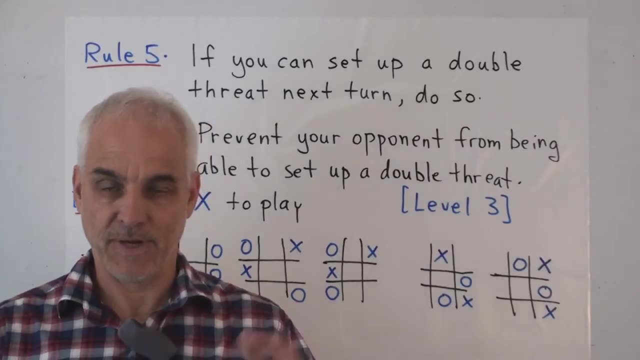 of making a double three so that they could win the time after that. So if you play this game a lot, you will become very quick at identifying possible threes. Direct threes are immediately visible, And then it doesn't take too long before you start becoming quite aware of double threats. 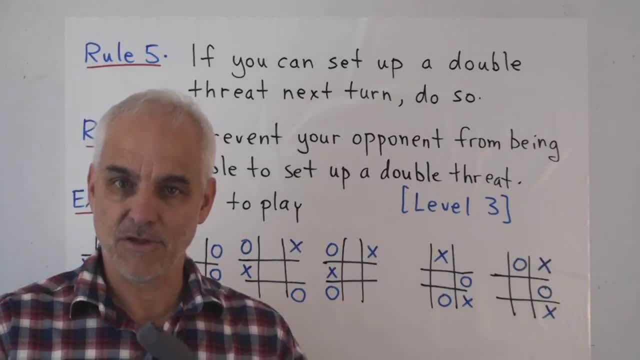 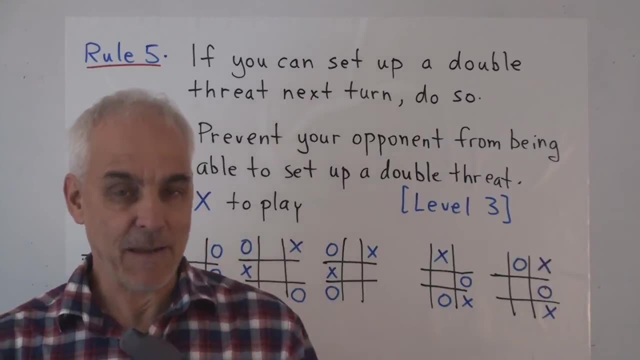 You can see immediately that there's a double threat move to be made by either player. There is then one further rule for further level of sophistication. We would go up one step and we look for a move which doesn't make a double threat. 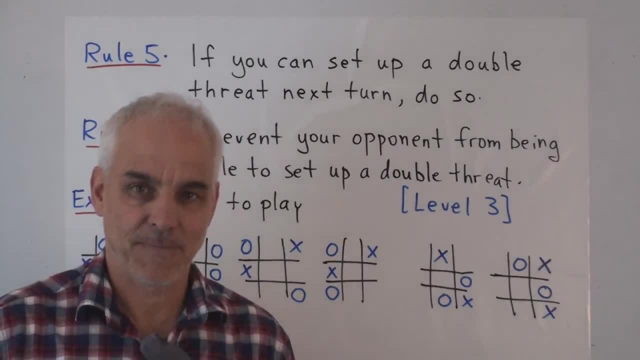 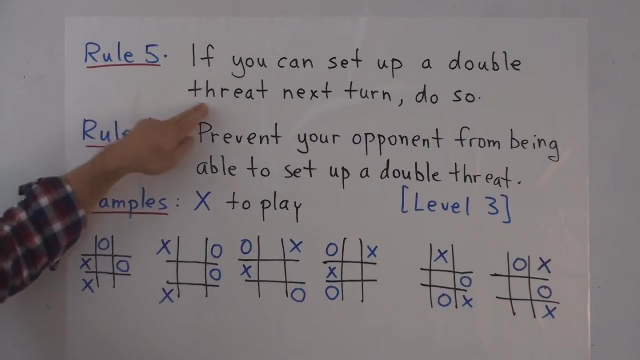 but which allows us to make a double threat on the next move. So, basically, it's a move that allows us to win, not this time, not next time, but the time after that. Alright, this is rule number five. If you can set up a double threat, next turn, do so. 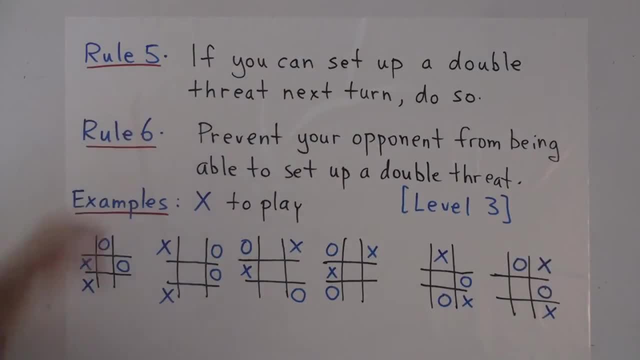 And the corresponding rule is that if you can't do that, make sure that your opponent can't, So prevent your opponent from being able to set up a double threat the time after his next move. This is level three strategy. So now we have a complete strategy in the sense that 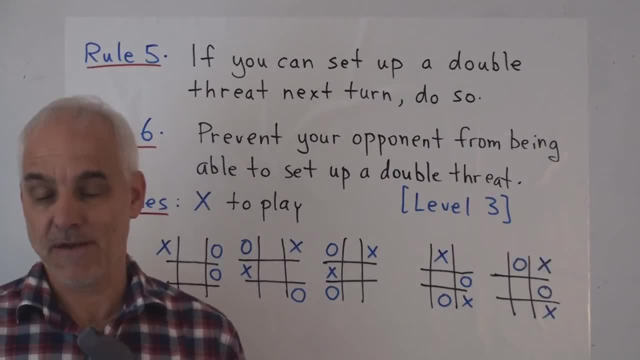 if you know these six moves, you will never lose at tic-tac-toe And you will win a lot of the time. Let's illustrate all six rules by a couple of examples. X is to play. It's our job to win. We are X. 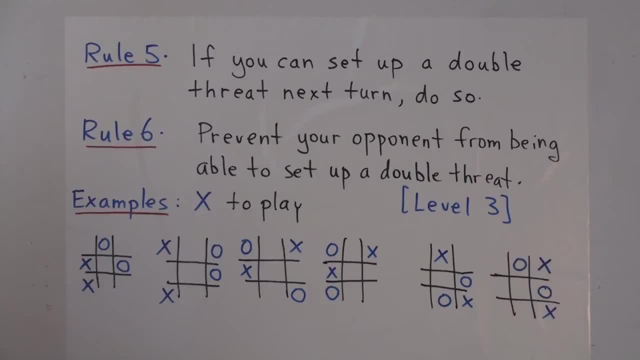 Okay, this is a very simple one. X is to play. Well, X had better play here, because that makes a three. So X wins. X wins immediately Over here. well, if you get sidetracked and you look at the two O's. 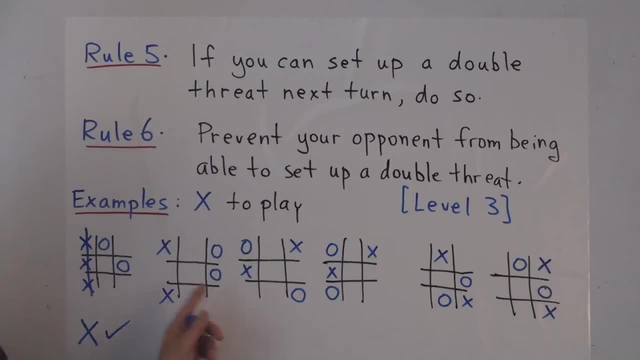 you might say: oh, I have to prevent the two O's from being made a three, But the first thing you should do is to look to see whether you can make a three and X can make a three, so he should play there and win. 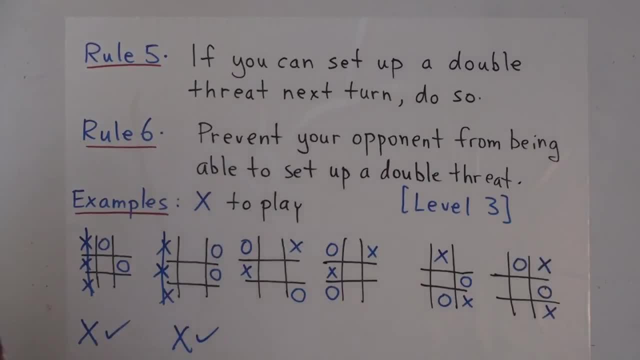 In this situation, rule number one doesn't apply, but rule number two does. X has to play here in order to prevent O from making three there. In this situation, X does not have a direct three, O does not have a direct three. 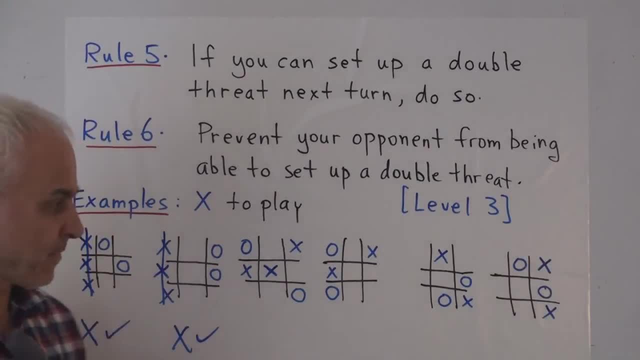 So X is free to think about making a double threat. Can he play somewhere that will threaten two, threes? Well, yes, there is such a place. Can you see where it is? There's actually one square that X should play on. 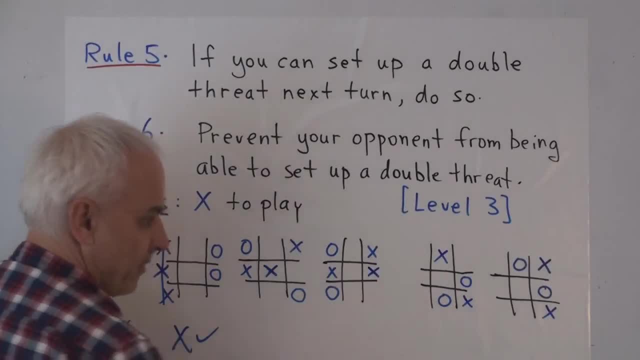 It's this square right here. That square threatens three in this direction as well as three in this direction. It doesn't matter which of those two. O plays to prevent, X will play the other one next time. So no, not O, X wins. 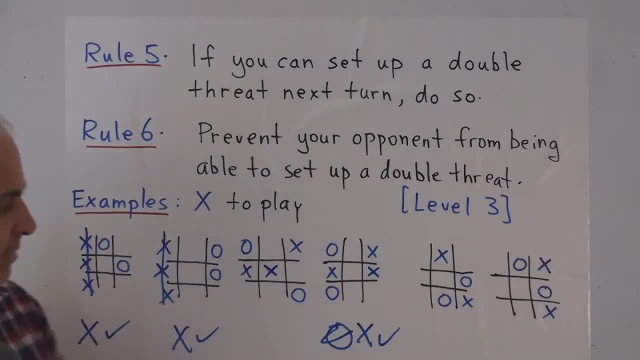 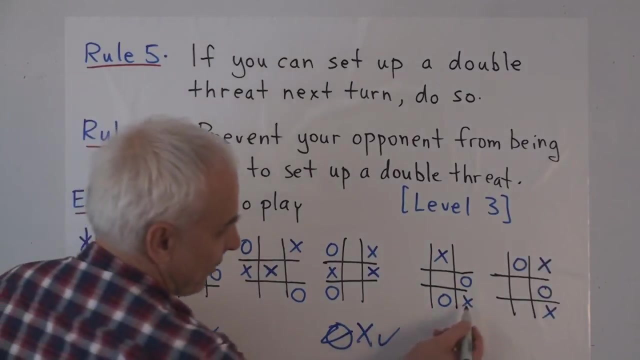 How about over here? Again, there's no direct win for X or O available. How about a double threat? Is there a place where X can play that threatens to make two, threes? Yes, there is Right there. Threatens a three along that row. 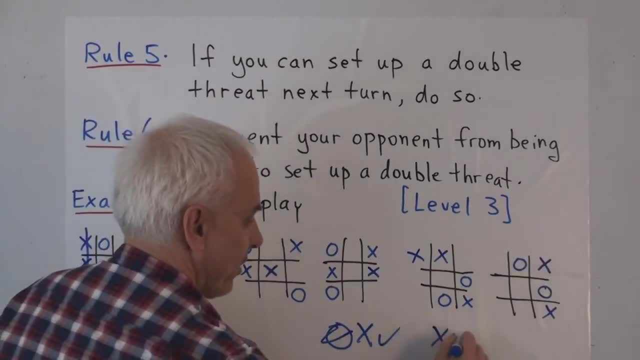 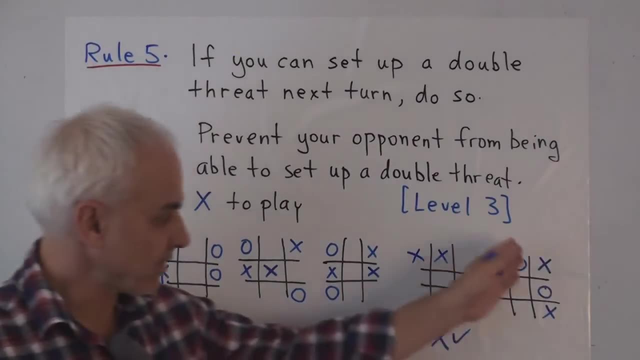 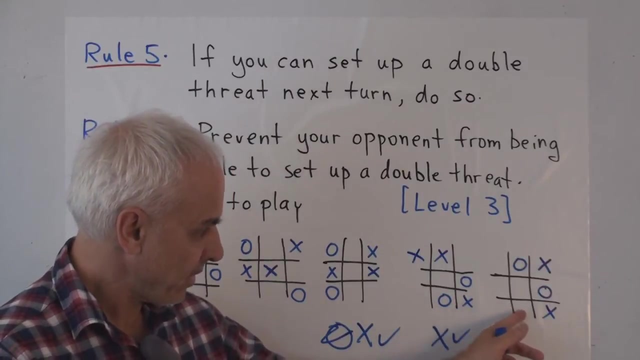 and also along that diagonal. So X is going to win here. And what about here? No direct three for X, No direct three for O. How about an indirect threat or a double threat? This won't do it. This will be a direct threat. 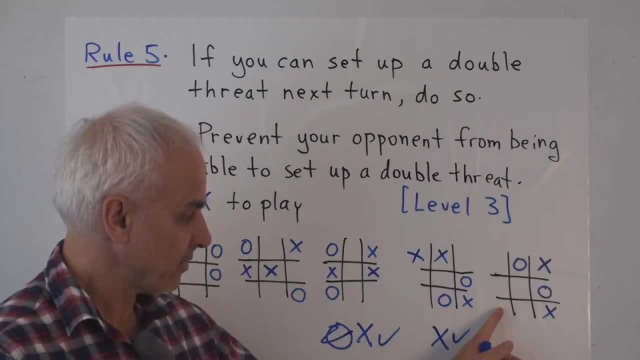 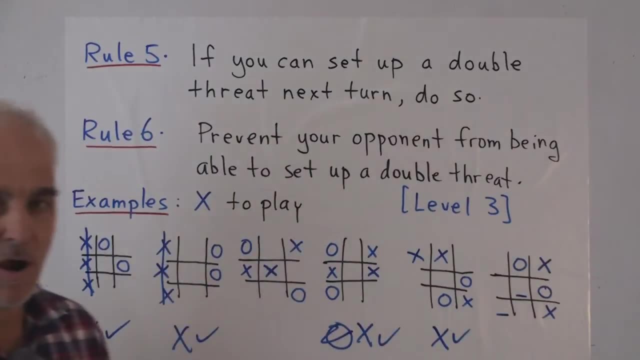 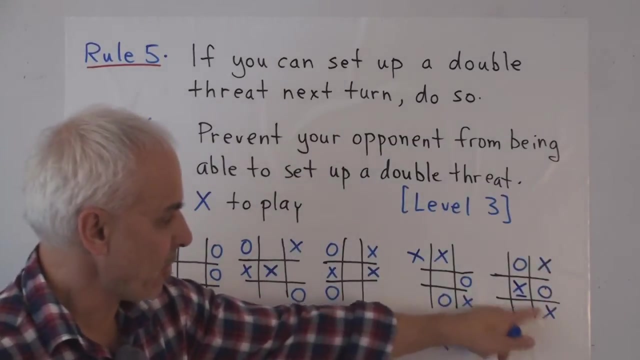 but not a double threat. This move will do it, But so will this one. So we have two possibilities. We can go either here or here. Both of them are double threats, So let's play here. That threatens three along that diagonal. 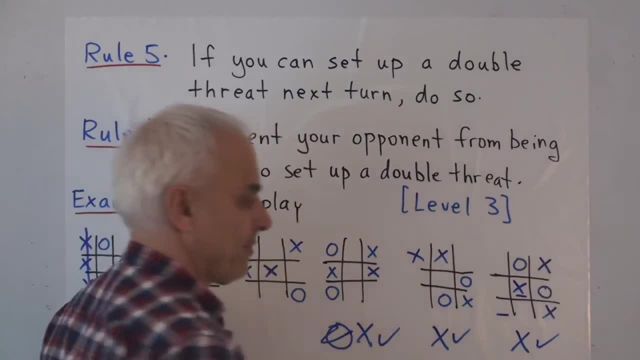 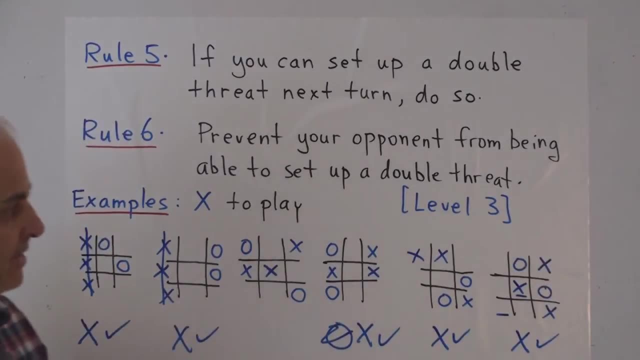 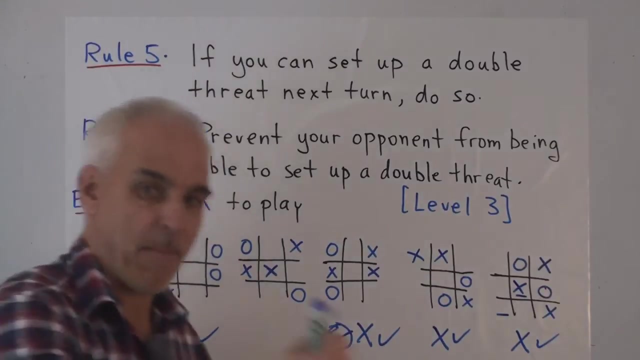 and also three along that diagonal. So X is going to win. So so far that's just the first four rules. Now let's have a look at this level three business. What does that mean when you go one step further and set yourself up for making a double threat? 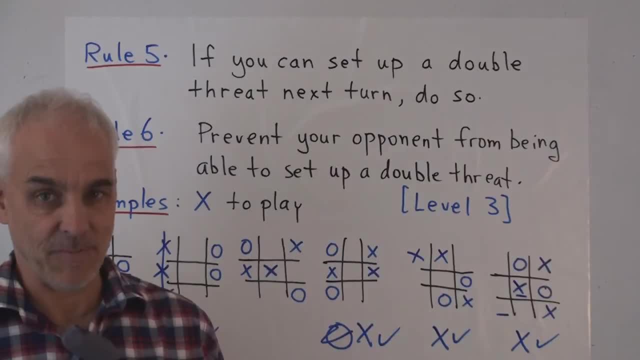 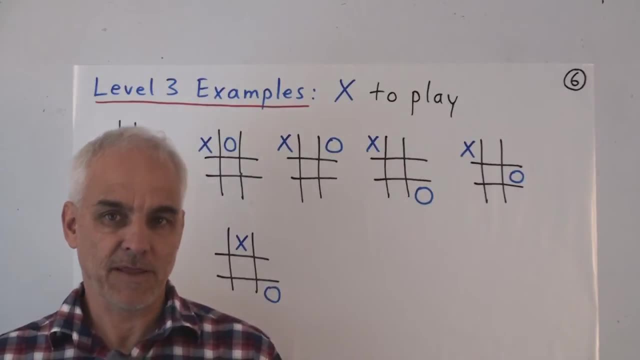 or preventing your opponent from setting themselves up to make a double threat. Okay, so here is level three play now, And the level three play starts pretty early in the game and has to do with these positions. So these are positions that you arrive at. 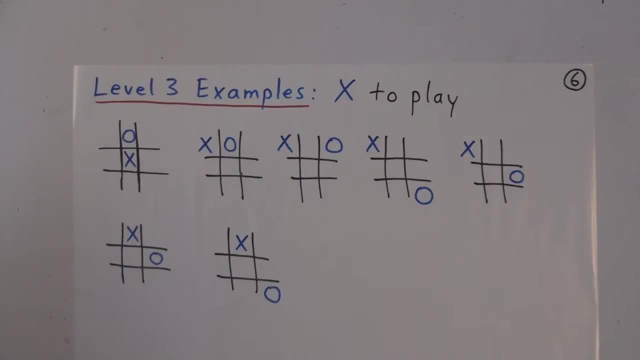 right after two moves. In the first move, X has played in the middle and O has made a mistake. O has played on the side, So X has played in the middle. How can she take advantage of O's mistake? She can't make three and she can't make a double threat. 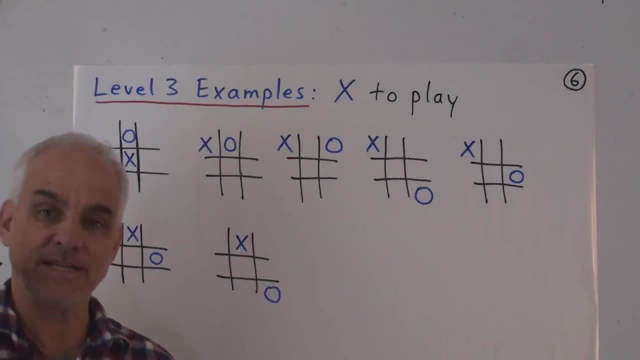 because she only has one X so far. But she can set up a double threat. And how can she do that? She can, for example, play here. That's a good move, because it forces O to play here, And now X is in a position to make a double threat. 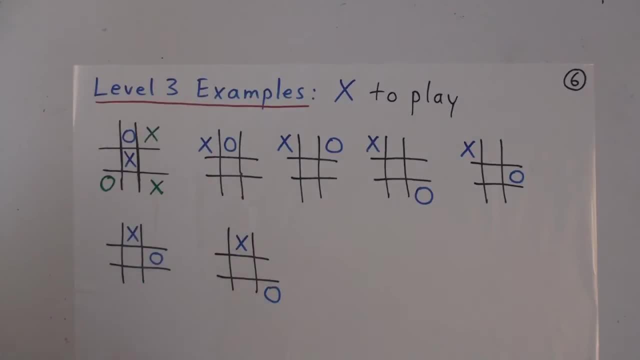 She can now play here, which threatens this three as well as this three, And there's nothing that O can do about it. So in this situation, X wins. So a very important consequence If X plays in the middle and O plays on the side. 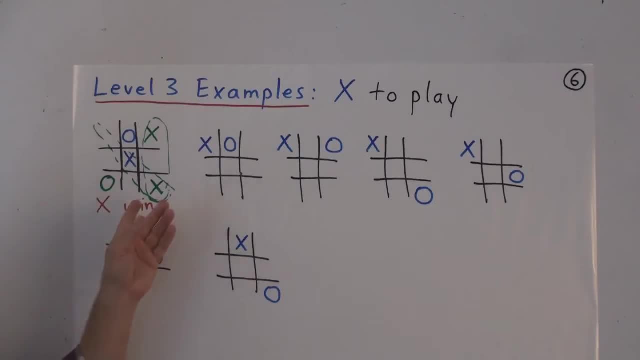 then X will win. if X plays this strategy And it doesn't matter which side square we're talking about- These four side squares, sort of in the middle of the sides, are all really the same, Just a rotation separates one from the other. 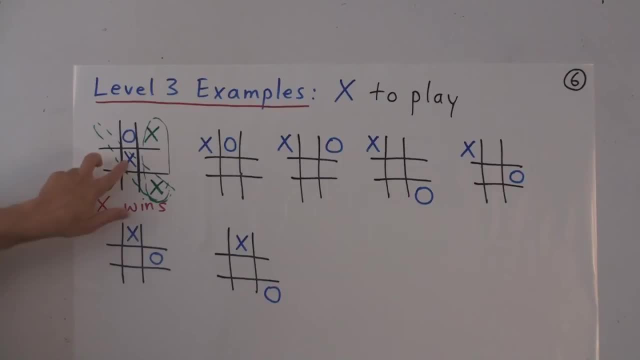 So if you understand the strategy in this situation, then hopefully you'll be able to translate it. when X plays here and say O plays there, X will still be able to force a win. Here's another situation where X wins, Where X has played in the corner and O has made a mistake. 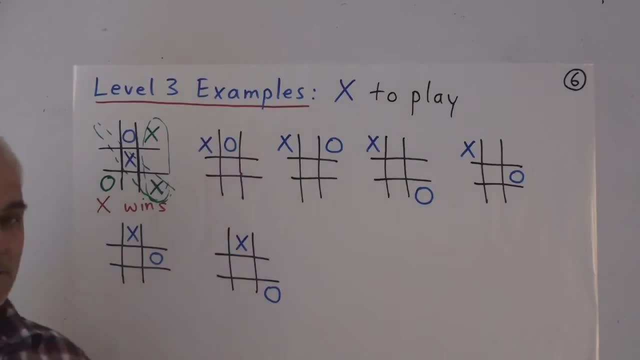 and played along in the side adjacent to X. What should X do? Well, X has a couple of different possibilities. One is to go here. In that case, O has to play here And now X plays there and has a double threat: here and here. 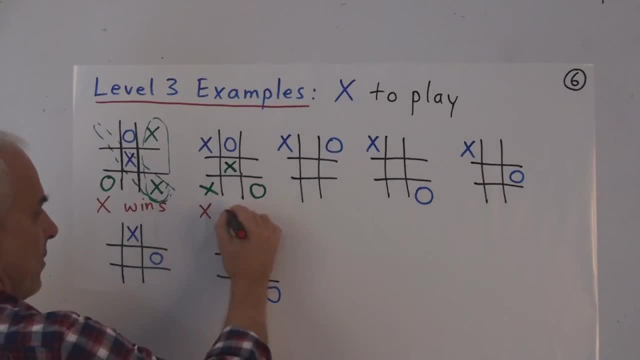 So X wins. You might like to work out the rest of these. before I do, You might like to pause the video, Just check to see what X's strategy should be in all of these cases, so that X wins for sure and O can do nothing about it. 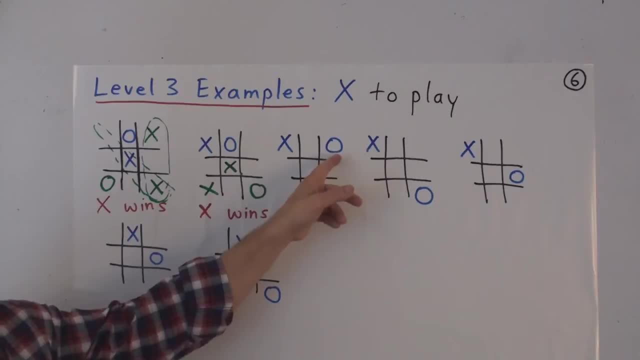 So in this situation, X has played in the corner and O has played in an adjacent corner. What should X do? X should play. Well, X has two choices: X can play here or here In one of the other corners, it turns out. 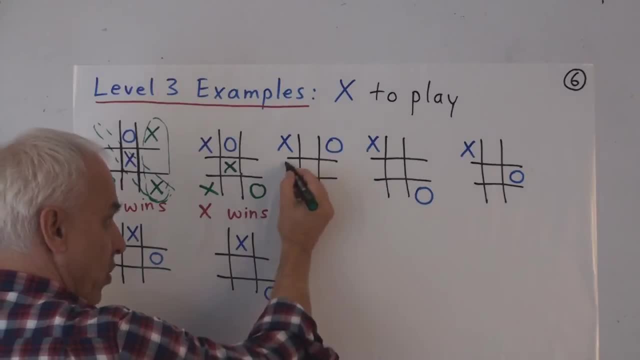 It doesn't matter which one. If X plays in this corner, then O will play here And then X can play in the other corner, making a double threat. X could also have played in this corner to begin with, in which case O would have been forced to play in the middle. 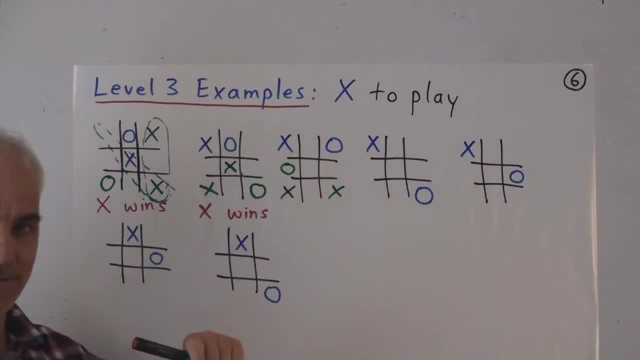 and then X could play still in the other corner, making a double threat. So if X plays in one corner and O plays in an adjacent corner, then X plays in the other two corners and wins. If X starts in a corner and O plays in the opposite corner, 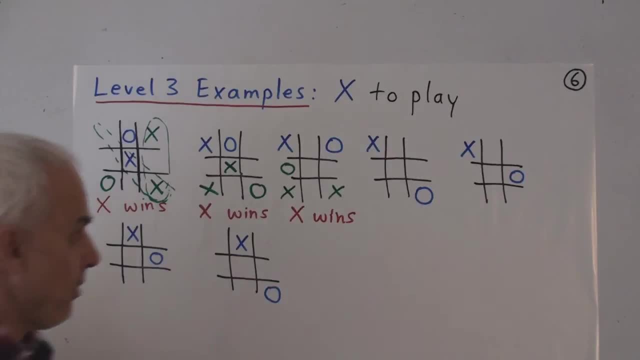 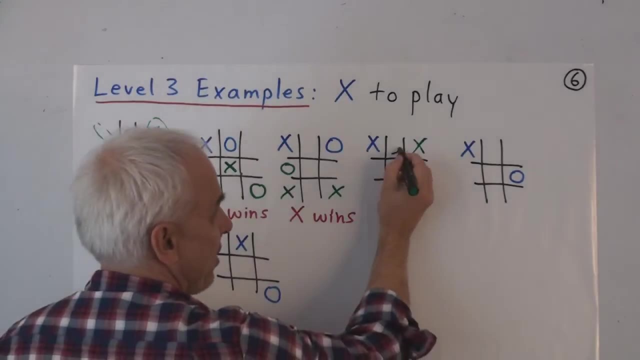 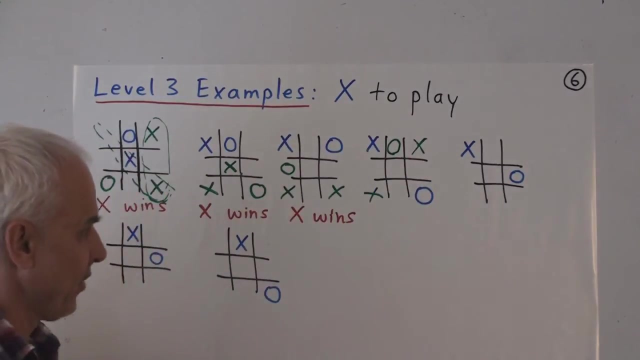 then what should X do? Well, X again should play in one of the empty corners. That forces O to play here, And then X can play again in the other corner, making a double threat. So X wins If X plays in the corner. 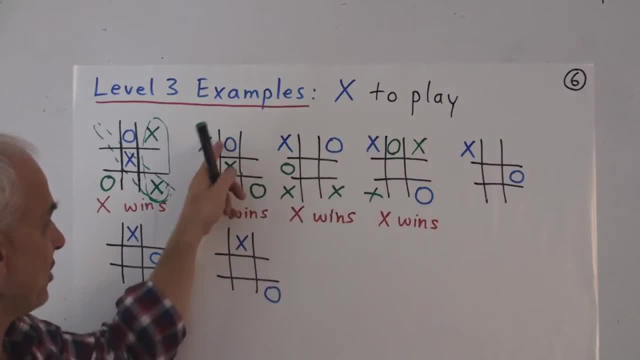 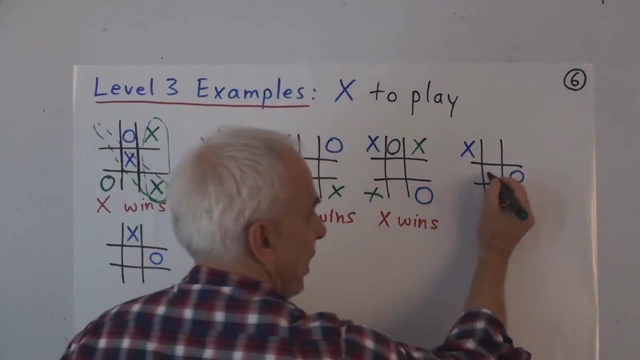 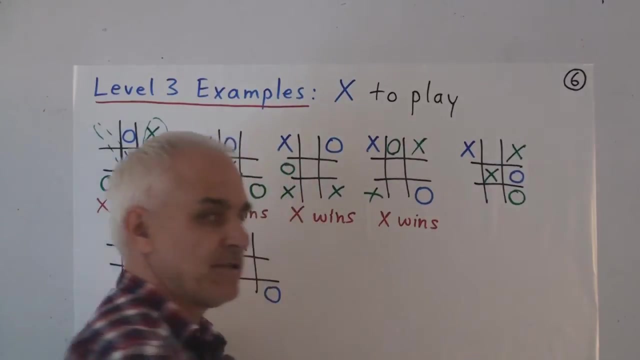 and O plays along the side, but not the side adjacent to X, but sort of the opposite to X. then what does X do? Well, X can play here, for example. then O is forced to play here, then X is forced to play where he wants to. 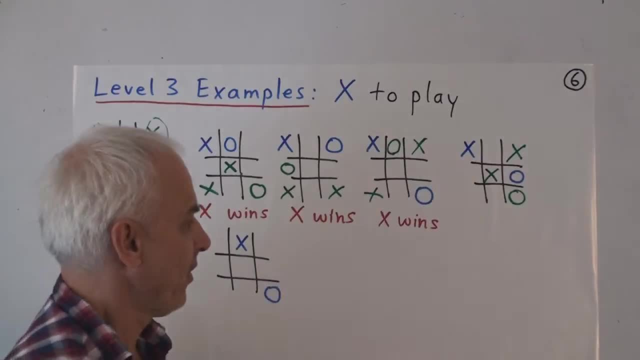 making a double threat here and here. so X wins, And in this situation X plays along the side this time, and O plays also along the side, sort of a side adjacent or diagonally adjacent. and then what can X do? Well, X can play in the center. 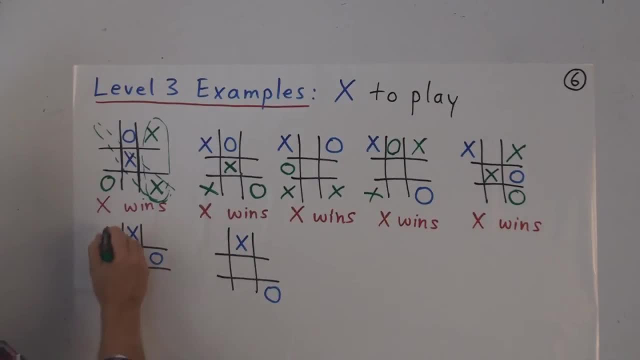 forcing O to play here. and then X makes a double threat there. so X wins. And finally, if X plays on the side and O plays in one of the opposite corners, then X can do what? Then? X can play here, then O is forced to play here. 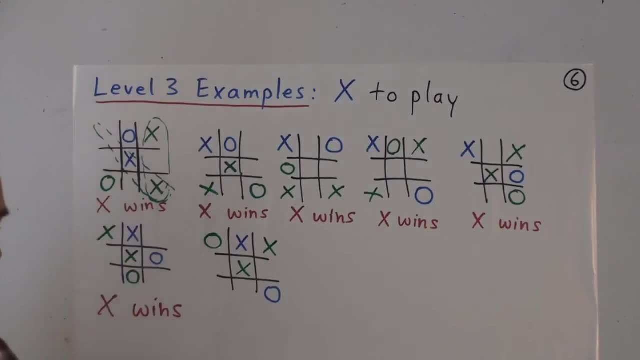 and then X is forced to play here, which is what she wants to do, by giving her a double threat, and so X wins. So this shows level 3 strategy on the part of X, showing how to use that rule number 5 If you can't make a double threat. 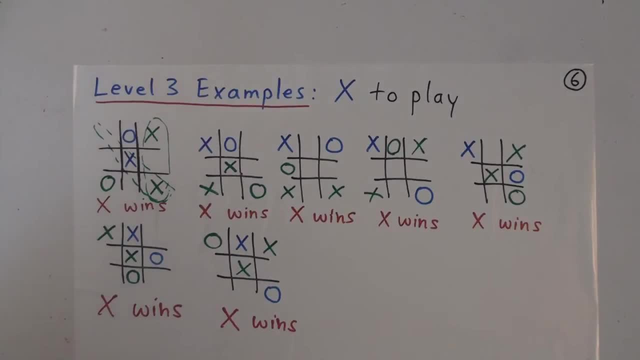 make a move that will ensure a double threat. And these positions that I've shown you here are also rather important because they teach you very important mistakes that the second player should not make. If the first player plays in the middle, then you do not want to play along one of the sides. 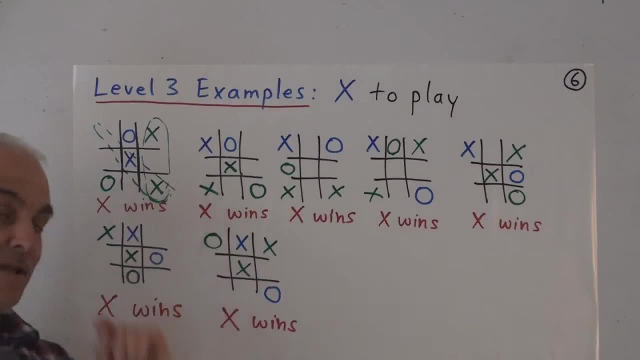 because if you do, then that gives X a chance to make a setup for a double threat. So if X plays in the middle, you have to play in a corner. Similarly, if X plays in the corner, then O cannot play along an adjacent side and O is also not able to play along the opposite side. 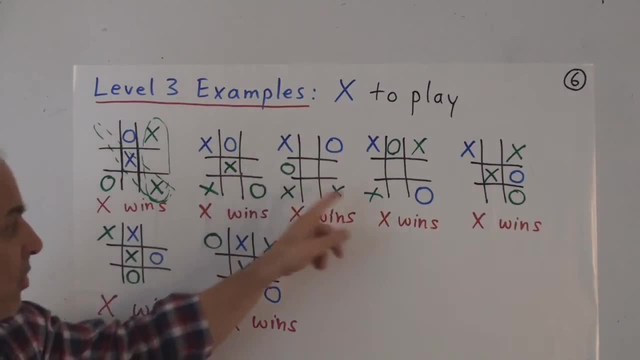 and he's also not able to play either in this corner or in this corner. So in other words, if X plays in a corner, then the only place for O to play is in the center. Otherwise O will lose And if X plays- a rather unconventional move. 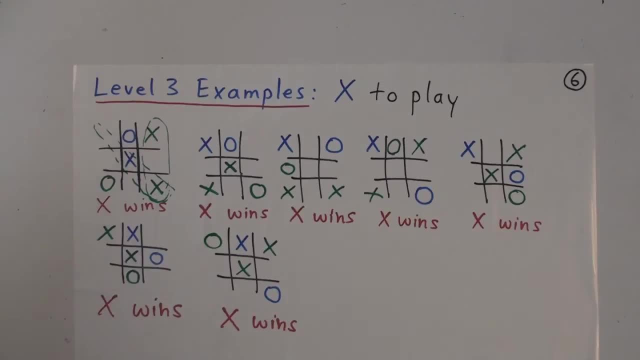 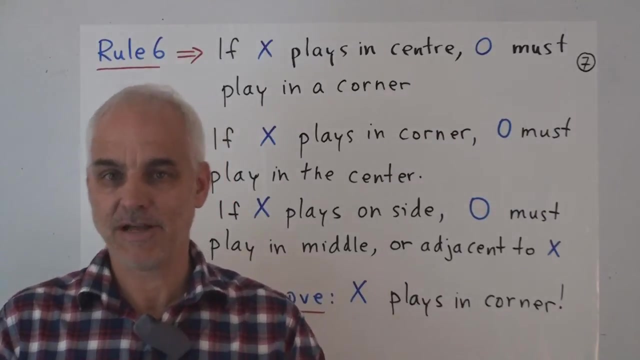 of playing along the side for the first move, then O must be careful. If O plays in one of these two positions, or in one of these two positions, he's going to lose. So rule number 6 says: prevent your opponent from being able to set up a double threat. 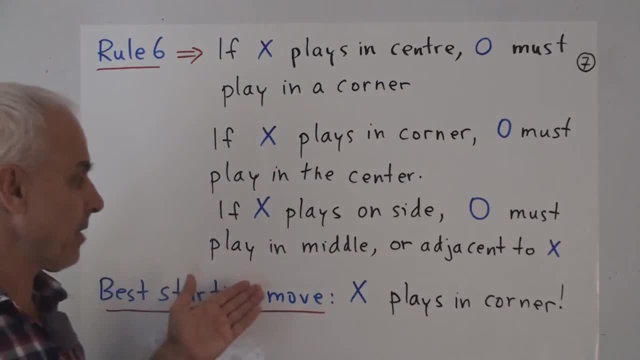 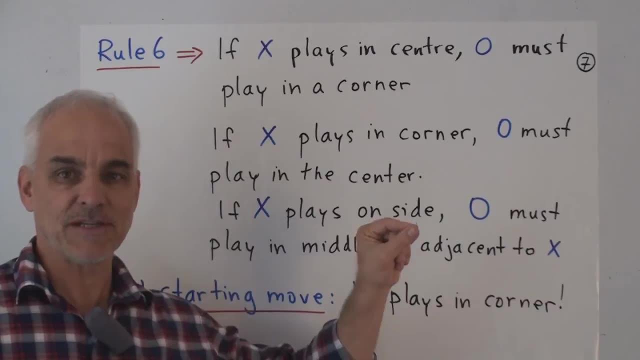 And effectively what that amounts to, are these prescriptions for O's first play? O wants to avoid the situations that we were talking about in the last slide, So if X plays in the center, O must play in a corner. If O does not play in a corner, 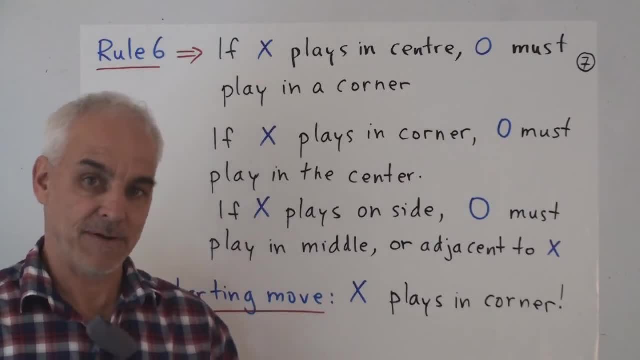 then X will be able to set up a double threat. like I showed you, If X plays in a corner, then O must play in the center. If he plays anywhere along the sides or the other corners, X will be able to play a set up move. 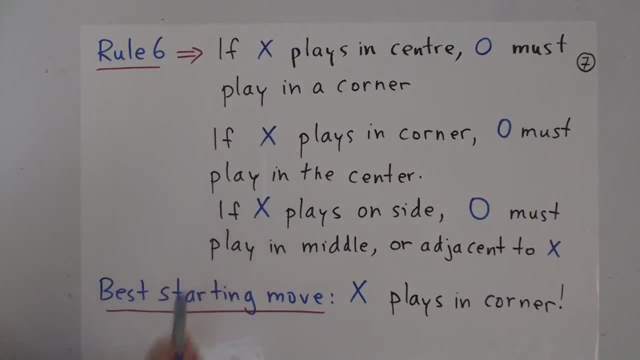 for a double threat. And finally, if X plays on the side, then O must play either in the middle or adjacent to X. If he plays in the other four positions, he's going to lose. And so, overall, what's the best starting move if you are the first player in a game of tic-tac-toe? 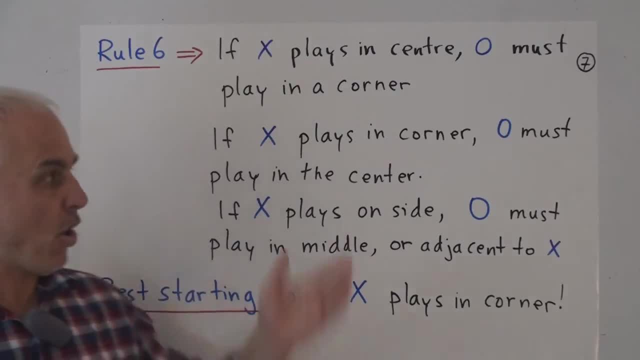 Well, it's a little bit of a matter of opinion. All three plays are valid. You're not going to lose if you play any one of those three moves and you play well. But if you want to maximize your chances of winning and you're playing a person who maybe is not such a good player, 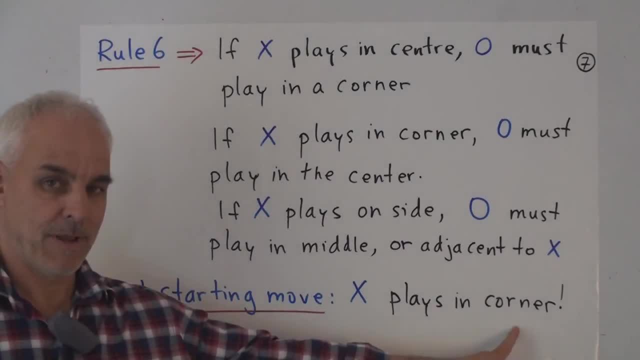 my suggestion is to play in the corner, Because when you play in the corner, you're putting O in this situation. You're putting O in the situation that there's only one move that will save him or her. She must play in the center. 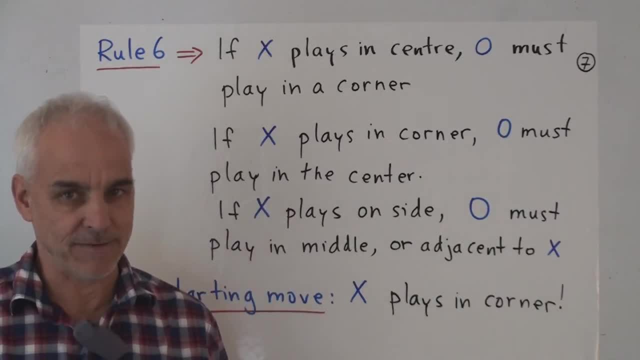 If she doesn't, you're going to be able to set up a double threat. So when you play in the corner, it allows your opponent the most number of ways to lose, Which is a good thing. So that's tic-tac-toe. 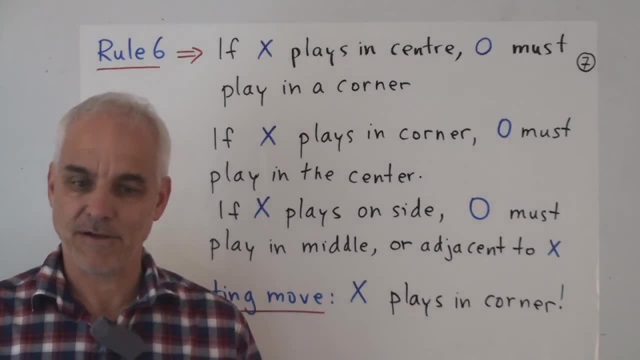 It's a little bit more subtle game than you might have thought And I hope you've enjoyed the somewhat logical presentation, The idea of looking one step ahead first, then looking two steps ahead and then, after we've mastered that, looking three steps ahead Each time we broaden our horizon. 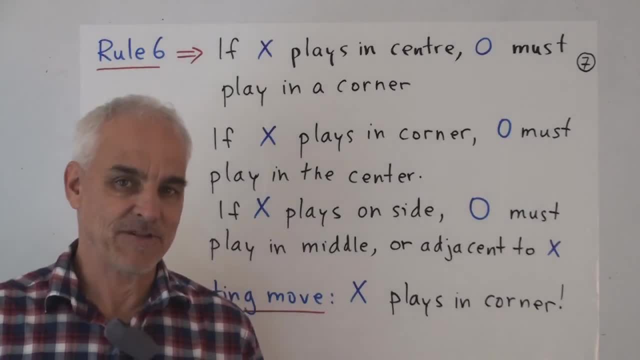 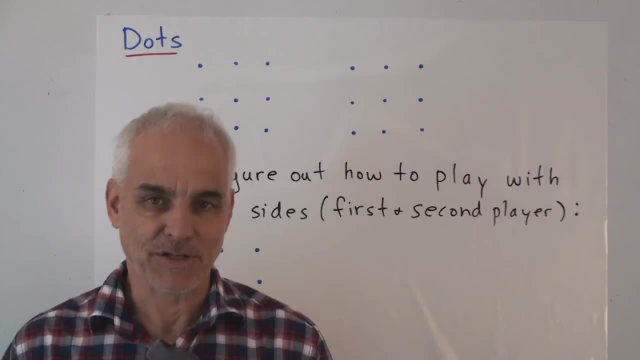 and we increase our power. Let's now have some games that you can experiment with on your own. So here's another famous game that's been around for a long time. I played it when we were kids. It's probably still a favorite. 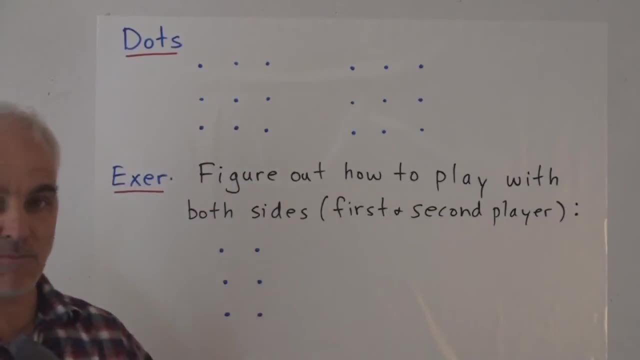 It's maybe just called Dots, And you have a bunch of dots arranged in a rectangular array And the size of the array is somewhat variable. The bigger the array is, the longer the game takes and the more complicated it is. Here's a relatively small version. 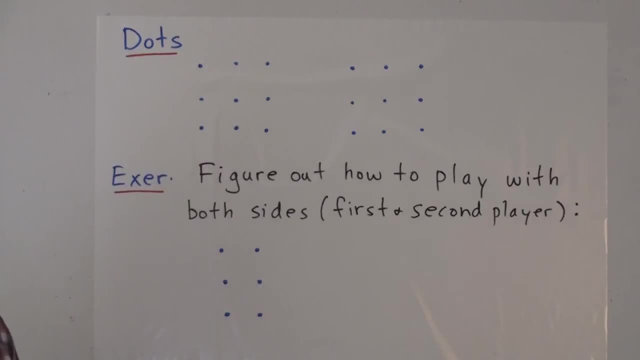 involving nine dots arranged in a three by three array, And the game is relatively simple. Both players take turns drawing a little connector between either two vertical or horizontally adjacent dots. Let's say the two players are A and B. Let's say A starts. 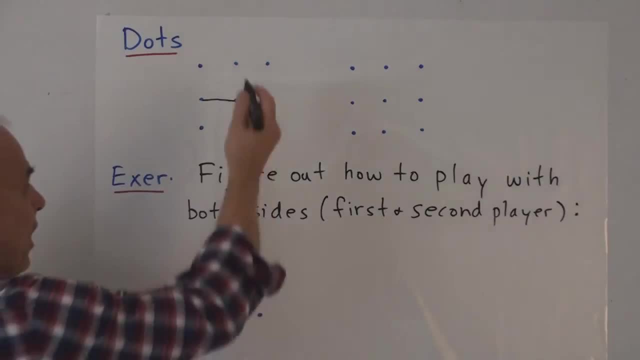 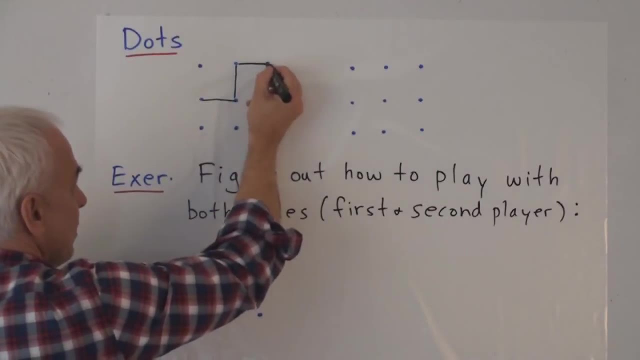 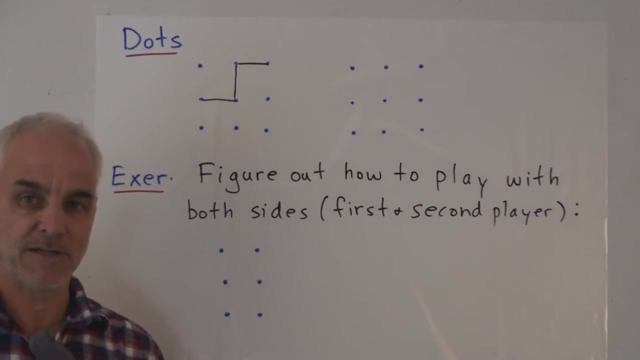 Joins those two adjacent dots And then B can use the same pen. maybe joins those dots And then A makes that connection. I should tell you what the aim is. The aim is to fill in boxes. Once you fill in a box, or make four sides to a box, 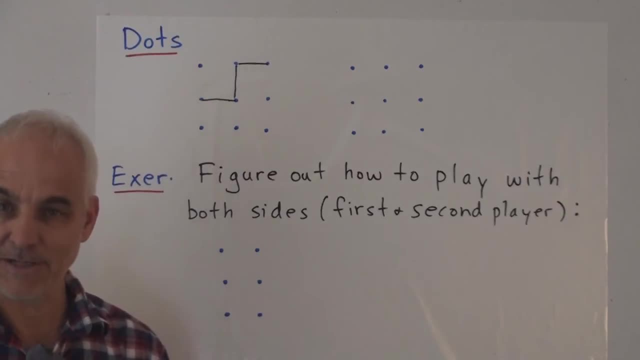 that box is yours, You put your initial inside that box and you get to go again. So when you complete a square or a little box, you claim that box and you get to go again, And the idea is to try to capture the most number of boxes. 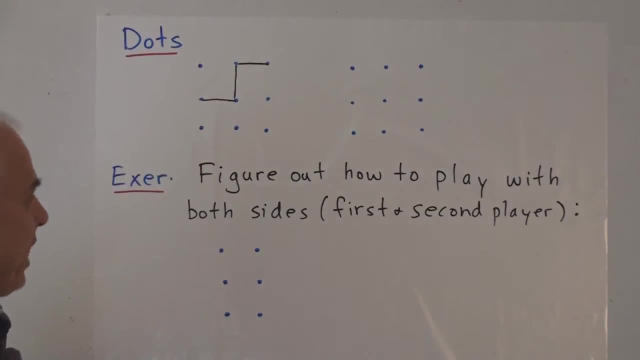 Alright, so we've had A and then B, and then A has played and, let's say, B now decides to go here. Oops, Maybe that wasn't such a good idea, because now A can close that box and put his initial inside there. Okay, so now A gets to continue. 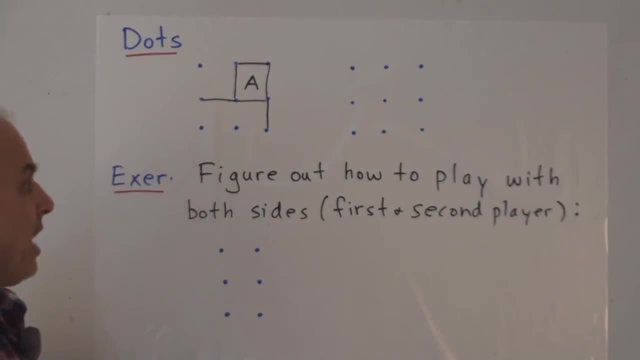 So A still has to play. Now it's B's turn B. oh, he's not going to make the mistake of doing that. He's going to go here instead. And that's not such a good idea, because now A is going to make that box as well. 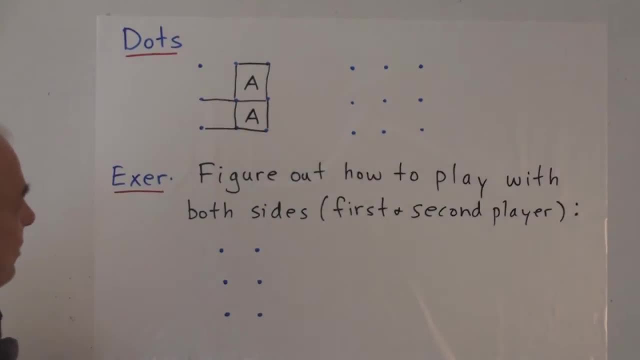 Now it's A's turn, And now A is forced to make a move like this, which allows B to finally get a box. But now B is forced to move and so he plays there and A gets to close off the last box. So in this situation, A wins. 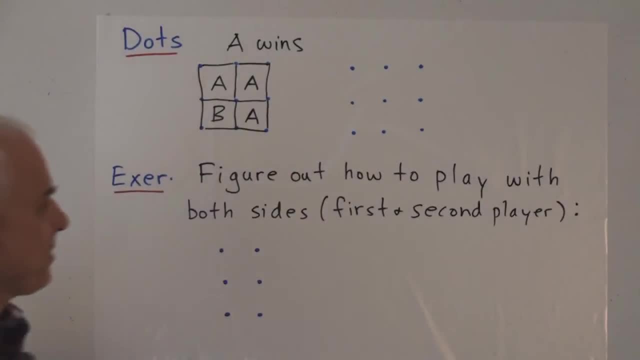 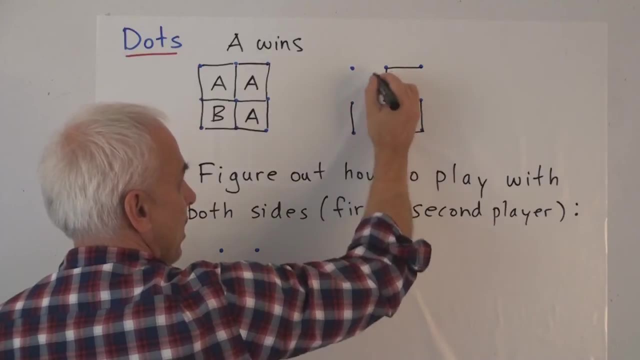 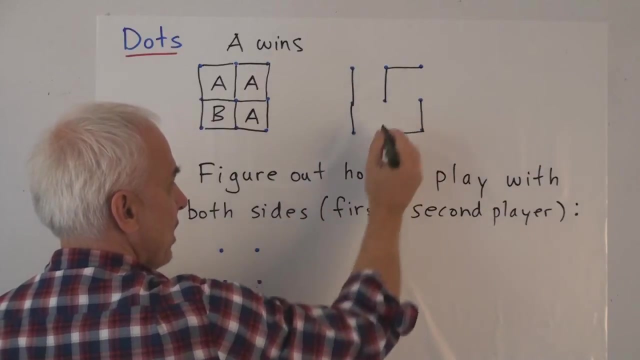 Let's play it again. A B A A, B, A, B A B. They're going to try to prevent a box from occurring until the last time. What was that? A B A, B A B. 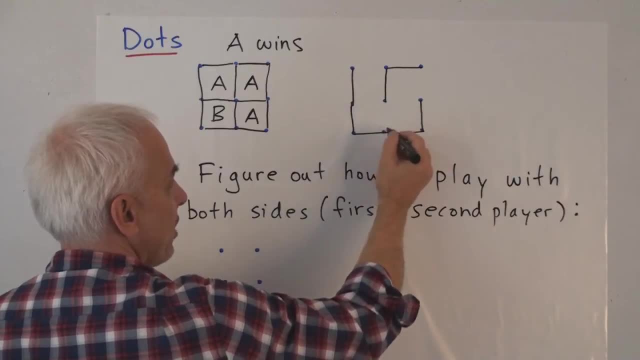 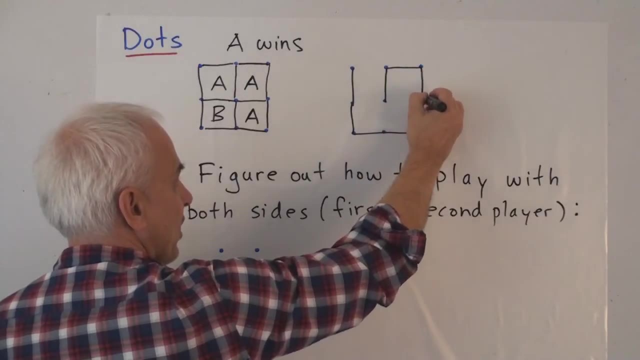 It's A's turn, A B, B is trying not to make a box. He looks like he's in a bit of a quandary. B goes here, But then A gets to make that one And then he gets to make that one. 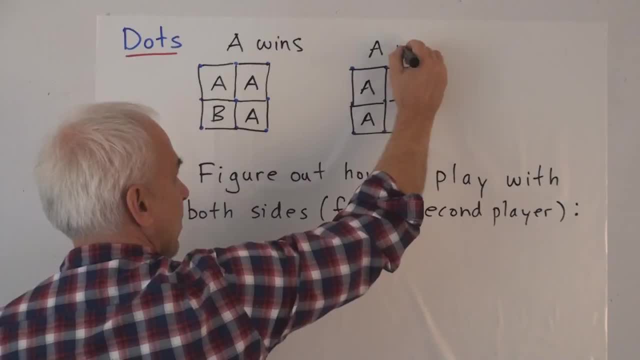 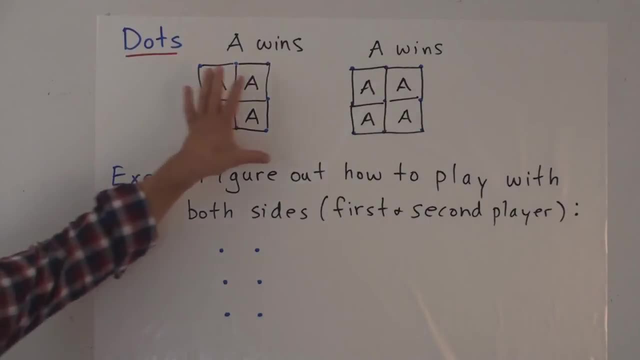 And then gets to make that one A wins again. Okay, so it's quite a demanding and challenging game when you have quite a lot of dots, But if you start with a small configuration it's easier to analyze. So your exercise is to figure out how to play this game. 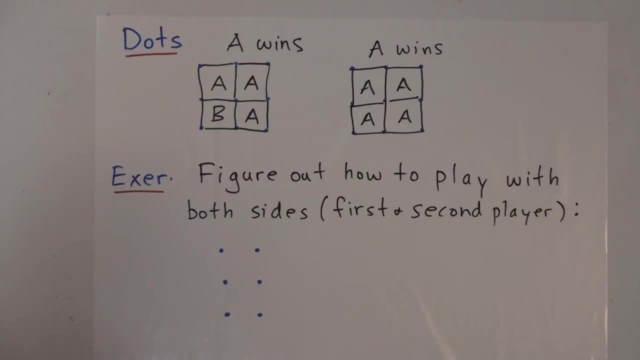 with both sides. So try to figure out the best strategy for both the first and the second player when we're starting with this relatively modest configuration of six dots. So there's going to be only two squares. You're fighting over two squares. The question is: what's the best strategy? 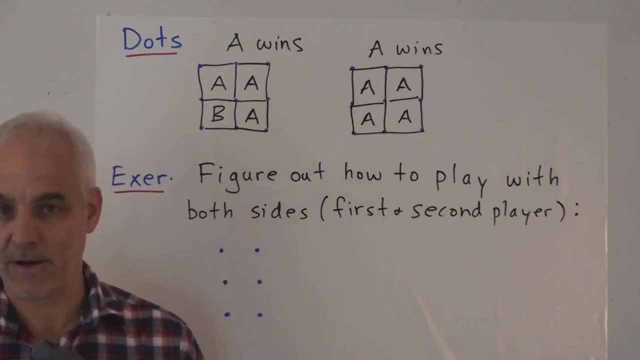 What's the best strategy for the first player? What's the best strategy for the second player? Suppose you had to play this game a hundred times next week and you were going to get $10 for every time you won. You would have to pay $10 every time you lost. 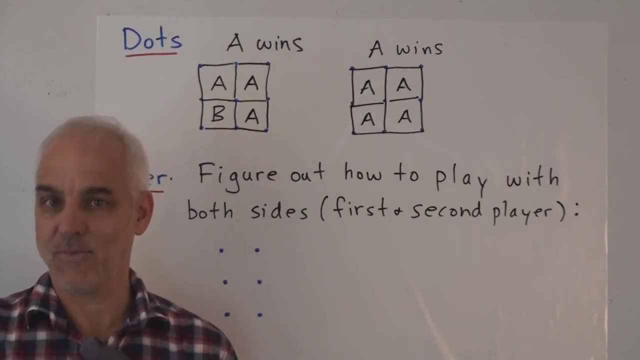 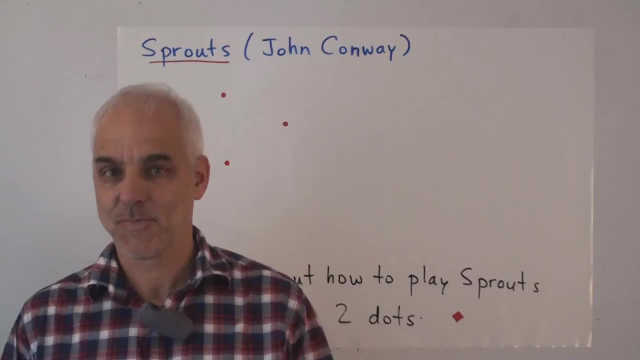 So you have to think ahead. What is the right way, the best way of playing this game? Quite a good exercise. And the second game that I want to show you is called Sprouts, And it was invented by a famous mathematician, John Conway. 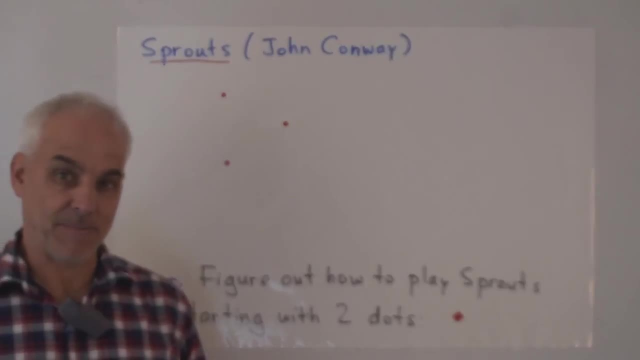 And it's a game played with a piece of paper and a couple of pens and some dots, And the more dots that you start with, the more complicated and longer the game is. So let's illustrate the game with three dots to start with. 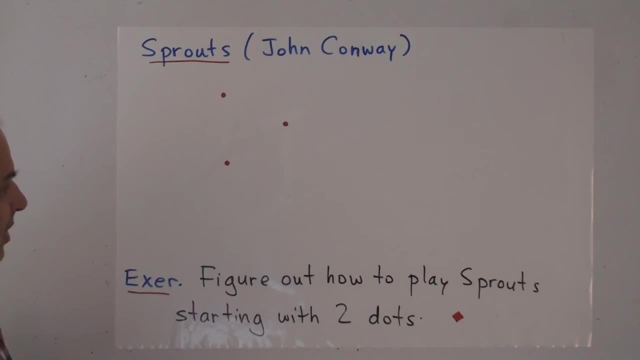 So the idea is that you want to join two dots with a line on a piece of paper, So not going off the paper and not going over any lines that you've already drawn. So let's connect this dot with this dot And when you make a new line, like that, 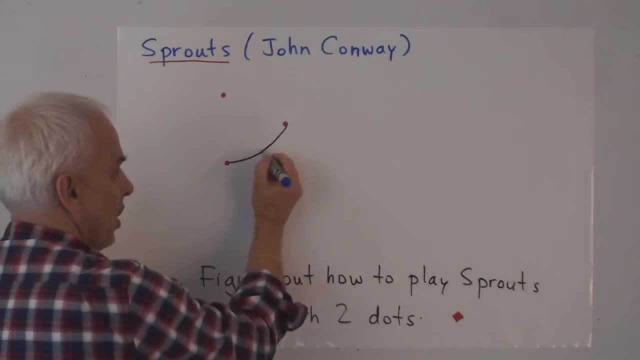 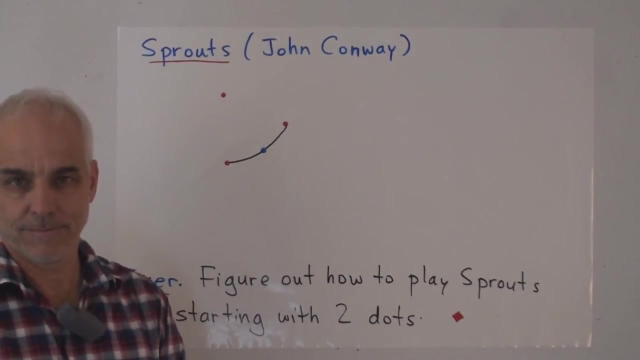 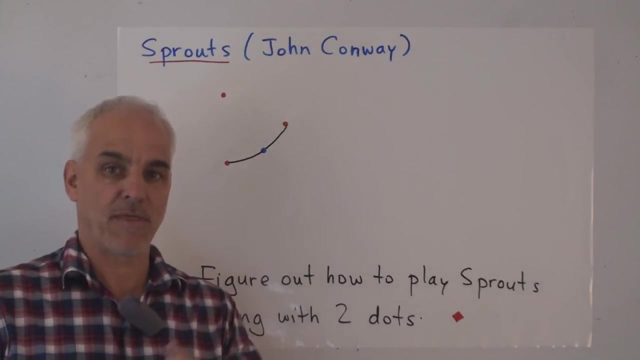 then out sprouts a new dot in the middle or somewhere on the line, Doesn't really matter where a new dot appears. Now the rule for these dots is that any dot can hold at most three lines coming out of it. So this dot at this point has one line coming out of it. 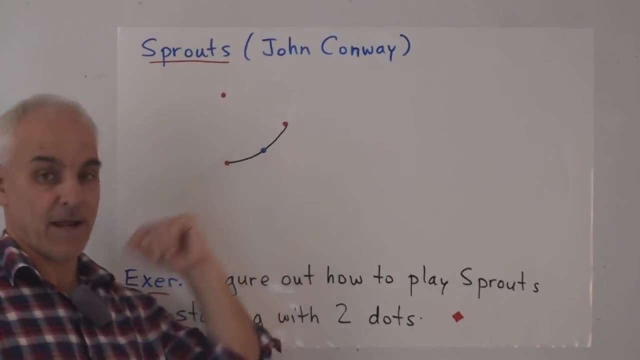 So does this one, And this blue dot that we've just made has two lines coming out of it. So three is the maximum number of lines that can come into any dot. So at the next stage, say the next player, he could connect this dot actually with itself. 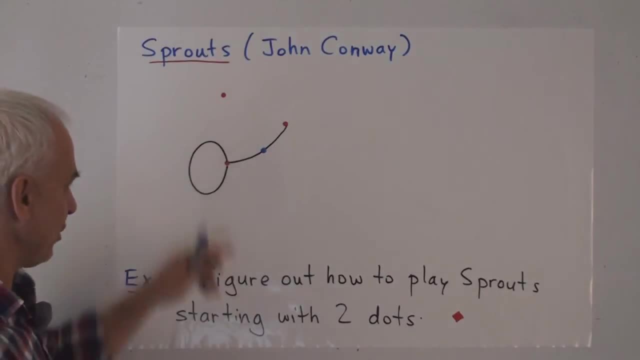 That's allowed. That's a loop from a dot to another dot And of course we have to make a new dot somewhere in the middle of it, right there. Now this dot is finished, So it can't be used anymore, But these other dots are still free. 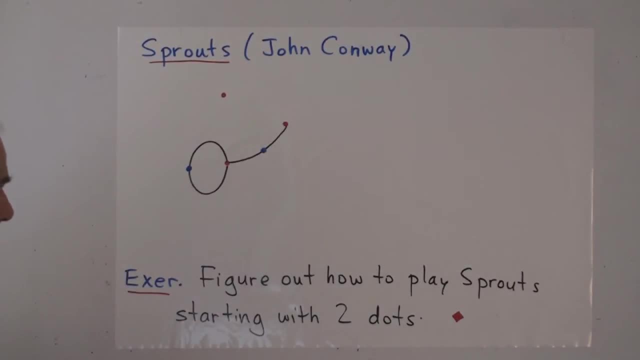 Okay, Well, and we keep going, And so the aim of the game is to be the last person who can make a move. If you can't move, then you lose, All right. So A has made that move, B has made that move. 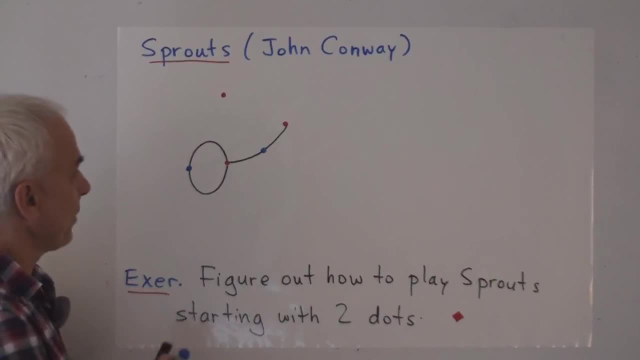 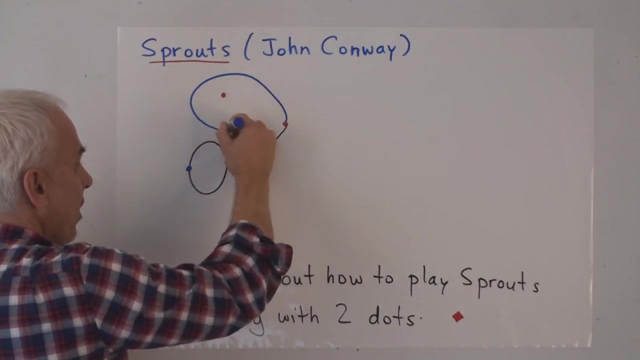 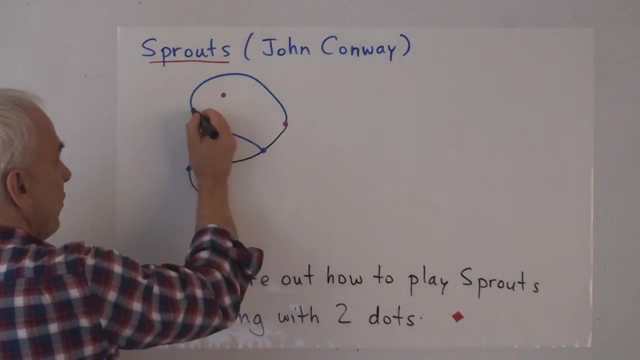 Now it's A's turn again. What will A do? Oh, let's say that A decides to go like this: Okay, And make a new dot, Another color. There's a new dot. Now it's B's turn. 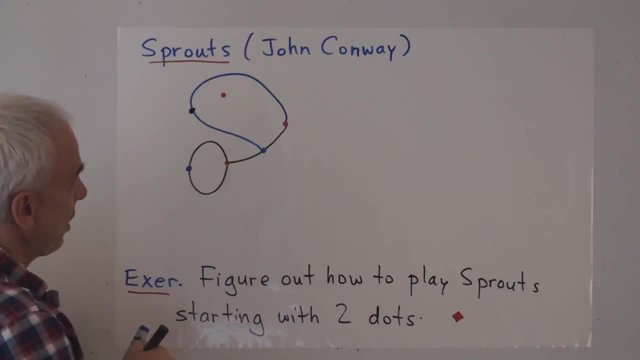 Well, B can join this dot with this dot, making a new line and a new dot. Now, how many dots are still in play? This one's still in play. This one's still in play. This one's still in play. 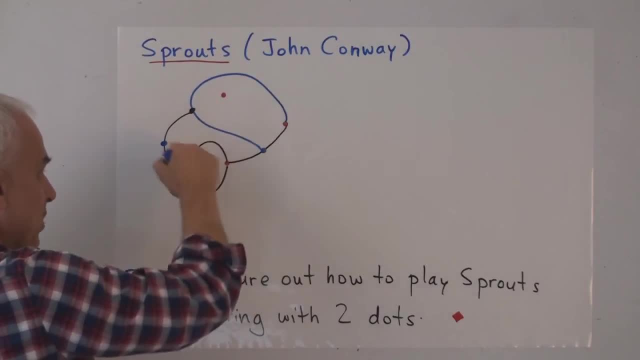 Now we've had A, B, A, B, And so now it's A's turn. Okay, A wants to be the last one to make a move. Okay, So what's A going to do now? Well, A is going to perhaps go like this: 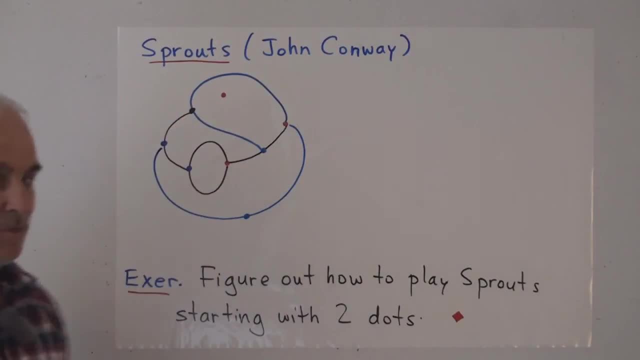 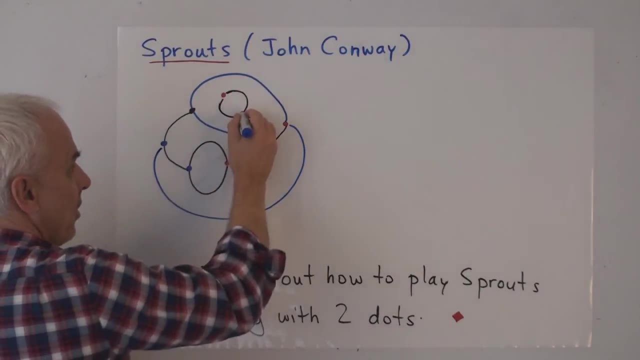 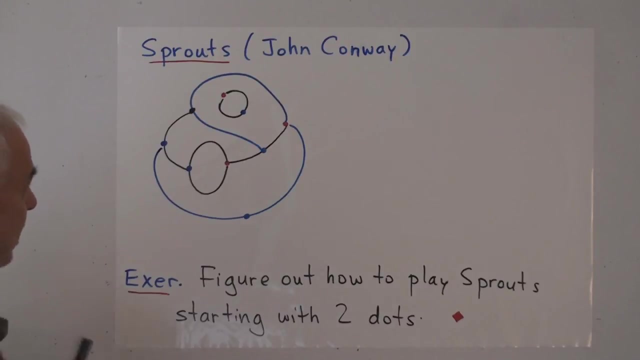 Connect these two and make a dot. These two dots can't be joined, though, But B can join this dot to itself, making a new dot, And now it looks like A is stuck, But no, there's one thing that A can do.